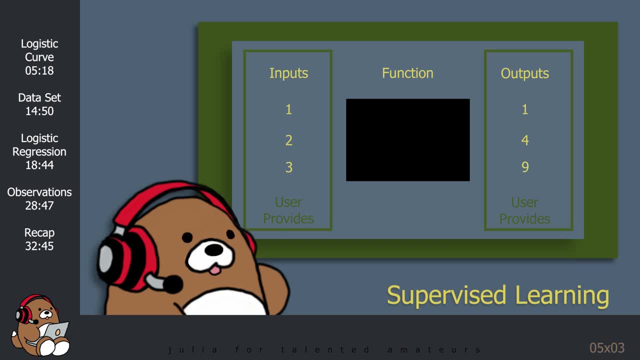 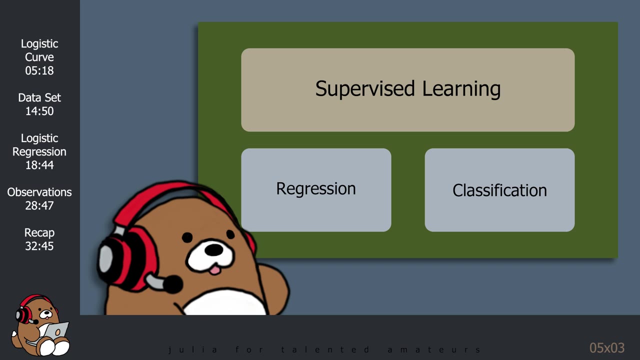 As a reminder, Supervised Learning is when the user provides both the inputs and the outputs and then the computer tries to estimate the function that determines the relationship between the inputs and the outputs. Supervised Learning may be split further between Regression and Classification. 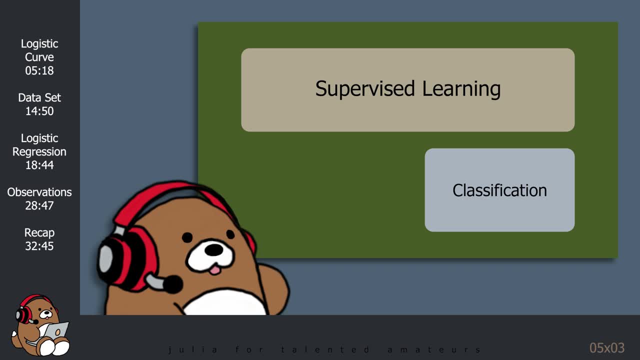 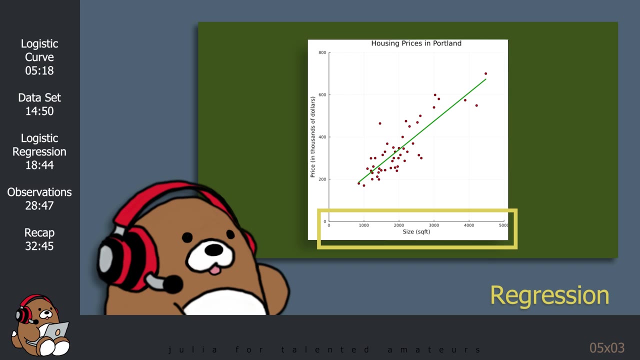 In today's tutorial, we'll learn about Classification. So how is Classification different than Regression? Last week we learned that Regression is used to understand the relationship between some independent variable x in order to predict the value of a dependent variable y. For a Regression problem, that relationship is said to be: 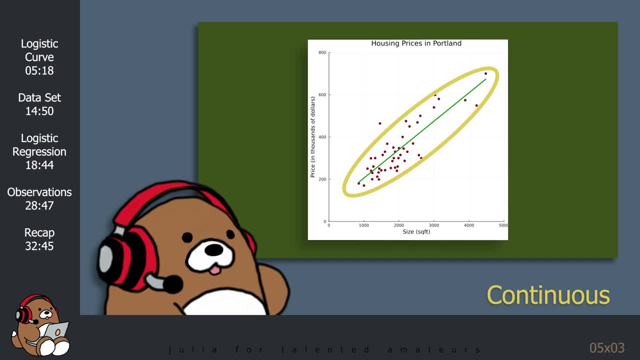 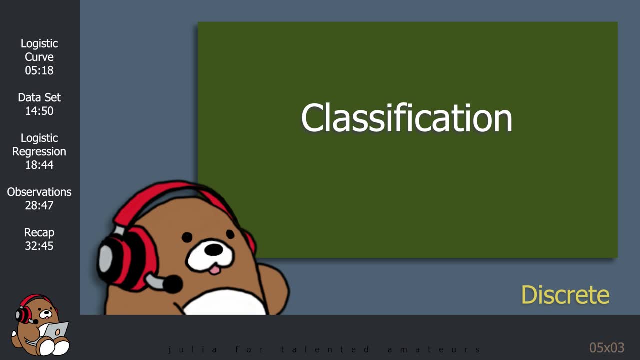 since for every value of x there's a corresponding value of y, Classification is used to predict a discrete value of y given a value of some independent variable x. The output in Classification problems is not continuous. Some examples of Classification problems include identifying whether an email is spam or not spam. 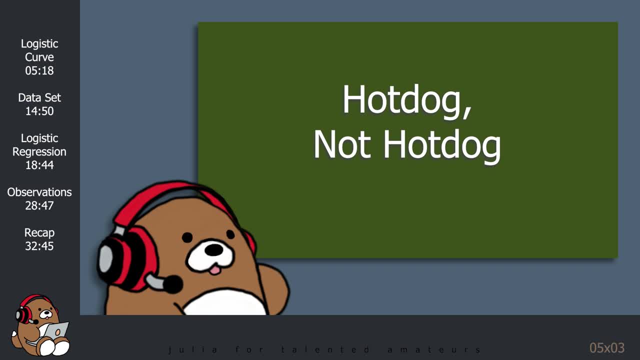 or identifying whether a tumor is malignant or benign. In these examples, there are only two possible outcomes for y: 1 or 0.. 1 represents a positive outcome, meaning that the email is spam or that the tumor is malignant. 0 represents a negative outcome. 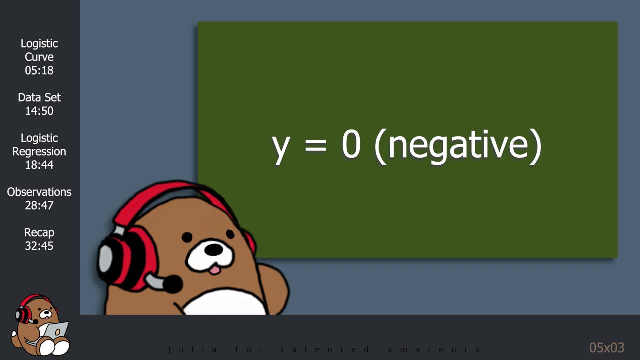 meaning that the email is not spam or that the tumor is benign. Here positive and negative do not have the same connotations as they might have in English, where positive implies something good and negative implies something bad. In machine learning, the terms positive and negative are used in a statistical sense. 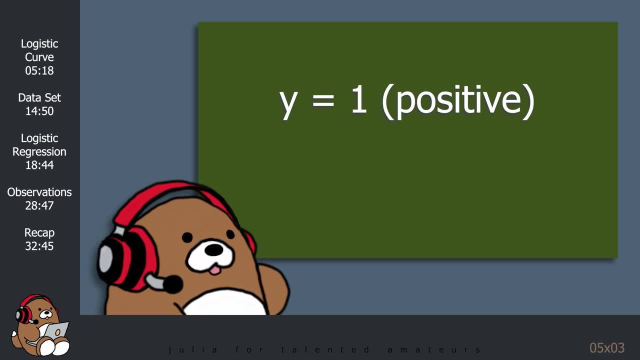 where positive means that whatever you're testing for has been found and negative means that whatever you're testing for has not been found. Classification problems with only two possible outcomes are known as binary classification problems. It's possible for a classification problem to have more than two outcomes. 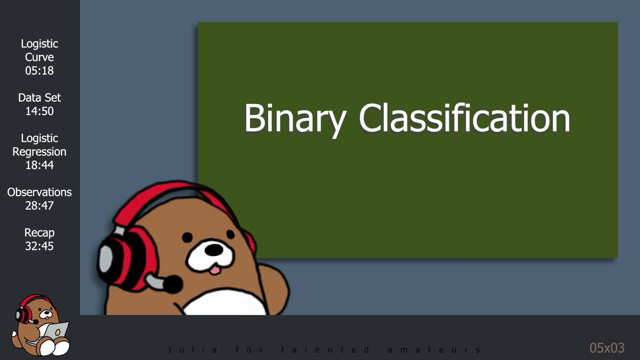 but since we're still learning the basics of machine learning, we're going to focus on a simple binary classification problem for today's tutorial. With linear regression we learn that there's a non-machine learning approach as well as a machine learning approach, But with classification there really isn't a 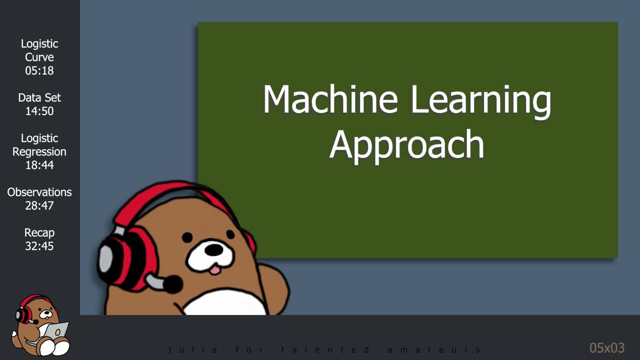 non-machine learning approach, so machine learning is the way to go. As a result, many real-world applications of machine learning involve some type of classification algorithm. By the end of this tutorial, you'll know how to build your own logistic regression machine learning classification algorithm to make predictions based on a binary classification. 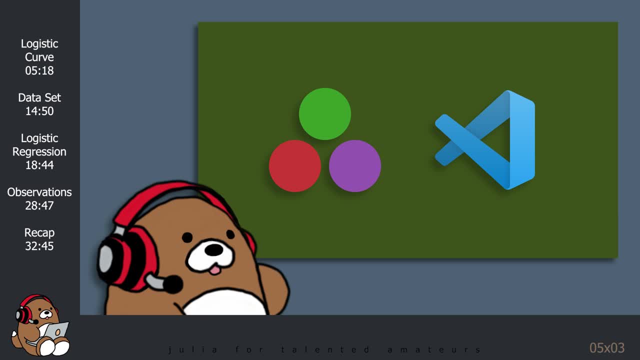 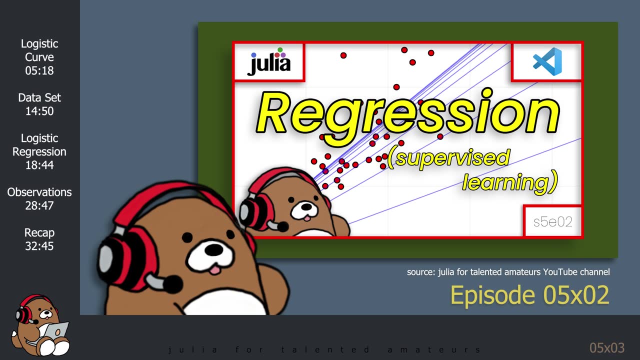 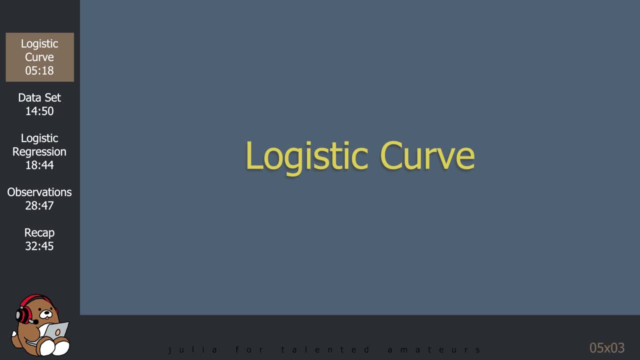 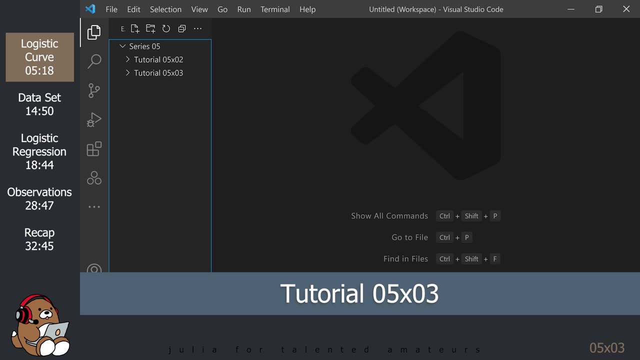 OK, let's fire up VS Code and get started. In your VS Code Explorer panel, create a new folder for this tutorial. In the tutorial folder, create a new file called sl underscore regression dot jl. Launch the Julia REPL by using Alt J, then Alt O. 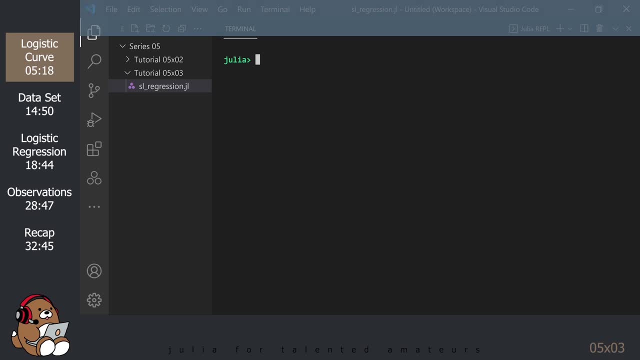 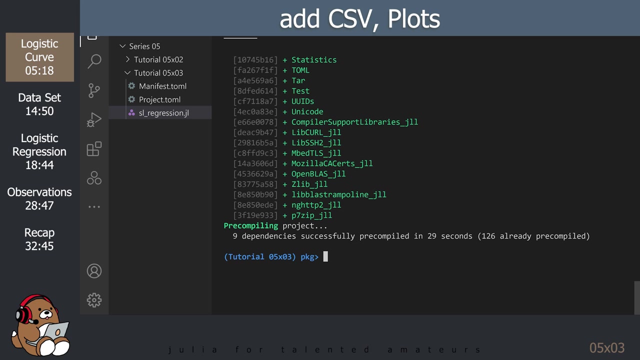 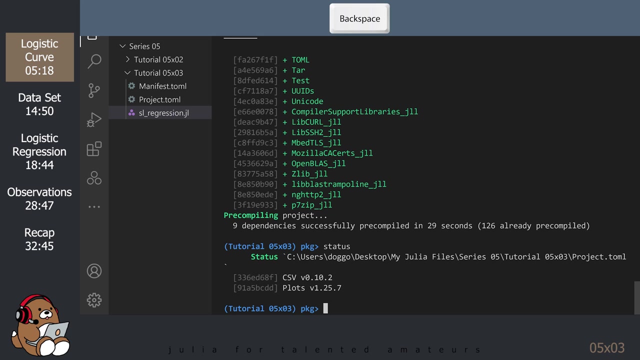 Maximize the terminal panel. Change the present working directory to your tutorial directory. Enter the package REPL by hitting the closing square bracket. Activate your tutorial directory. Add the CSV and PLOTS packages. Type in status to confirm the version numbers. Exit the package REPL by hitting backspace. 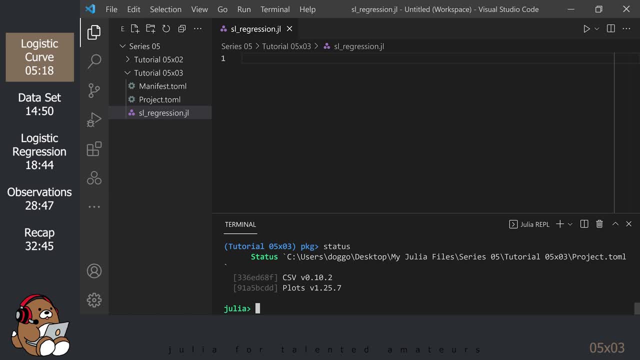 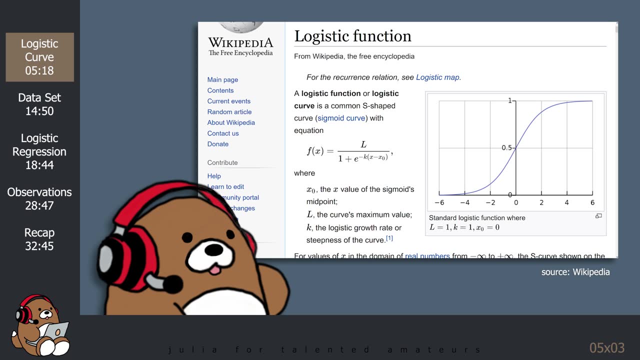 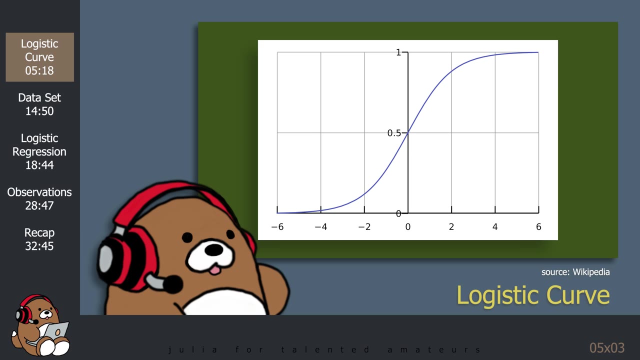 Click Save- Minimize the terminal panel. Before getting to the machine learning algorithm, let's take a look at the logistic curve. As you can see in this Wikipedia article, a logistic curve has a distinct elongated S-shape starting from zero on the Y-axis- when x is negative infinity- and then crossing the Y-axis. 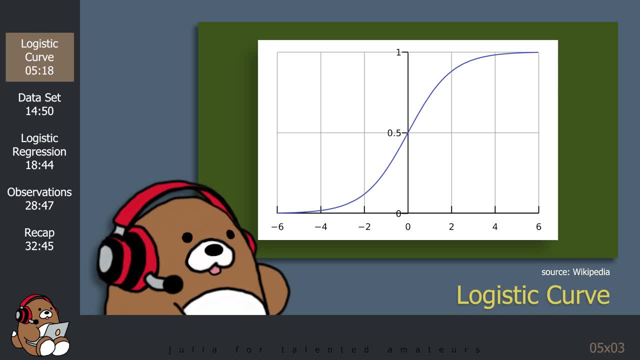 at 0.5, and then going to 1 on the Y-axis. on the Y-axis. This is now easier to understand if you're using some kind of algorithm that would be suitable for this대k to be used for this program- to 1 on the y-axis when x is positive infinity. This logistic curve is also known as the sigmoid. 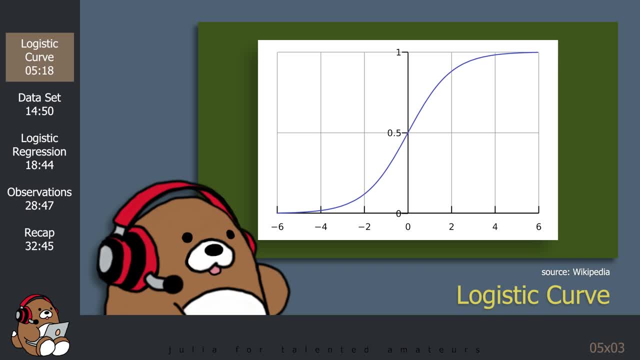 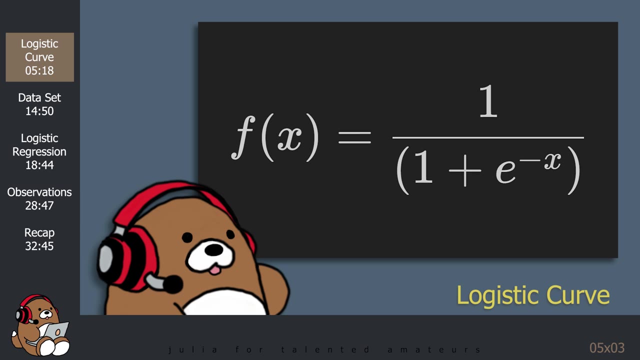 curve. Unlike the straight line that we use to solve linear regression problems, a logistic curve will always have an output that falls between 0 and 1 for any input That scripted E in the equation for the logistic curve is Euler's number, which is like the less. 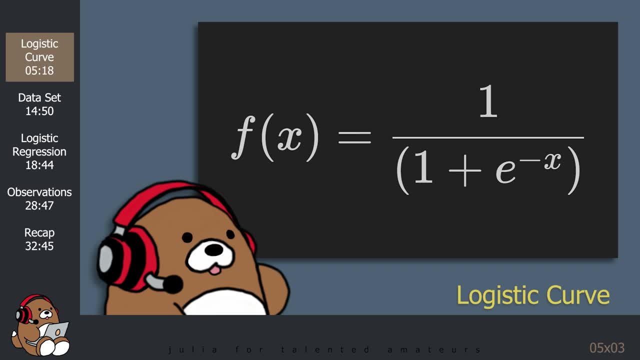 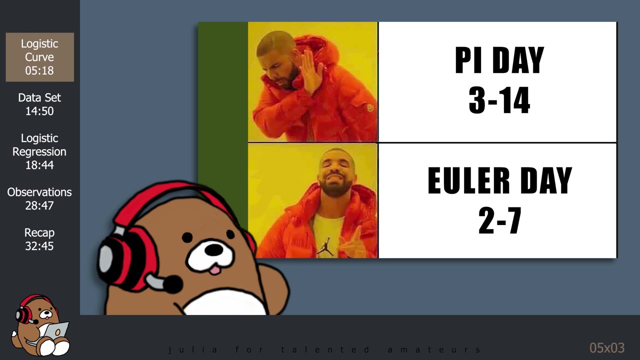 popular version of Pi. in the world of mathematical constants, Euler's number has a value of approximately 2.718.. While everyone celebrates Pi Day on March 14th, sadly no one celebrates Euler Day on February 7th. The logistic curve is also known as the logistic curve. This logistic curve is also known as the. 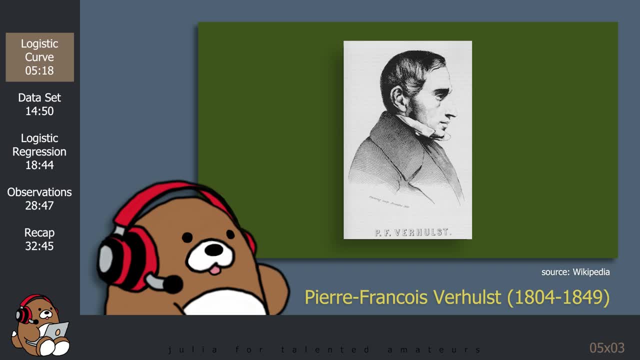 logistic curve. While everyone celebrates Pi Day on March 14th, sadly, no one celebrates Euler Day on February 7th. The logistic function has been around since the 1800s. It was introduced by Pierre-Francois Verhulst, who was a Belgian mathematician, who used it to explain the stages of population growth. 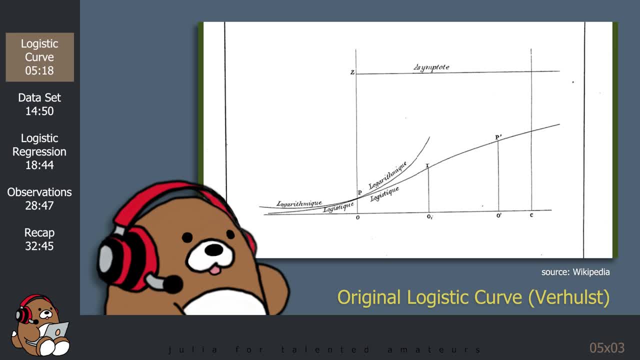 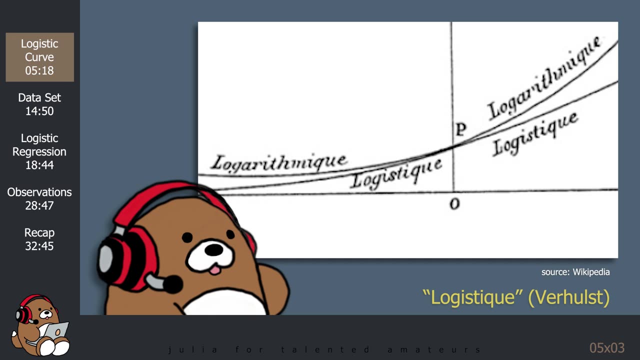 with the initial stage growing exponentially and the later stage slowing exponentially until the population levels off at some saturation value. It's a mystery as to why he used the term logistic to describe this curve, But the term has survived and so it's still being used today. 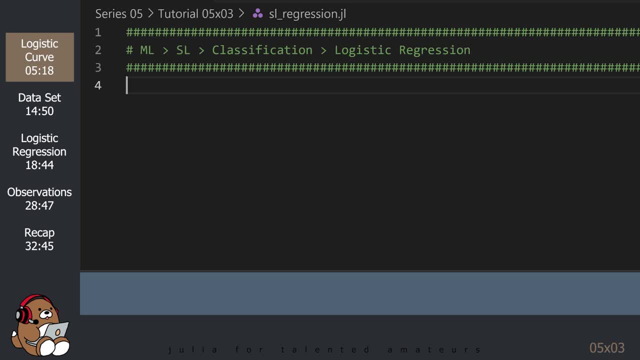 Let's use the Plots Package to generate our own plot of the logistic curve so that we can become more familiar with it. This is the same version of the logistic curve that was in the Wikipedia article. EXP is a built-in Julia-Wilk-Wilk combination of the logistic curve and the logistic curve. 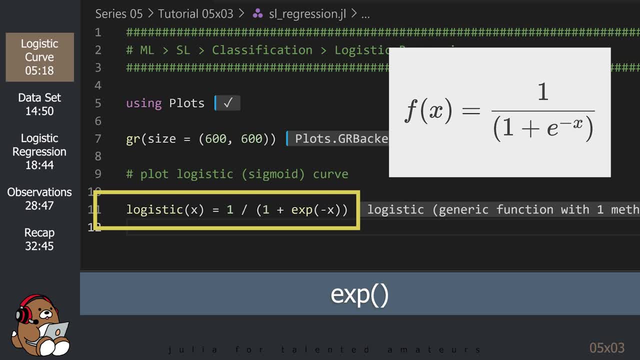 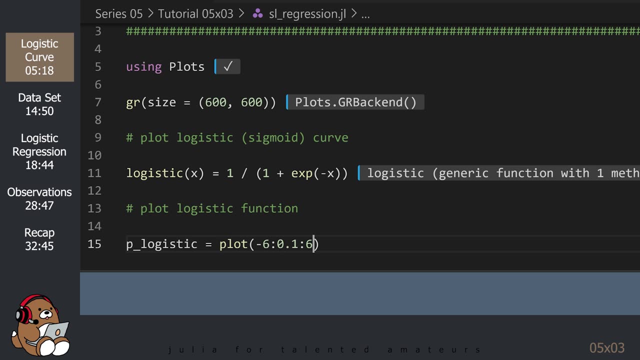 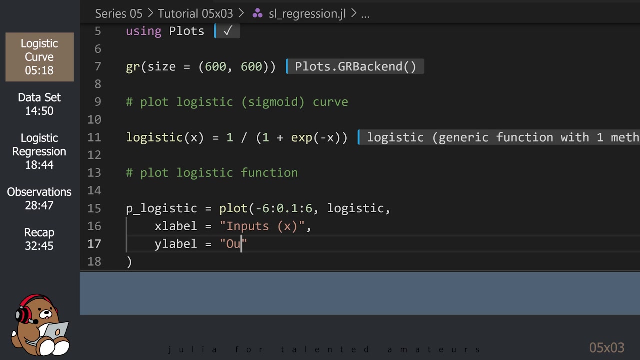 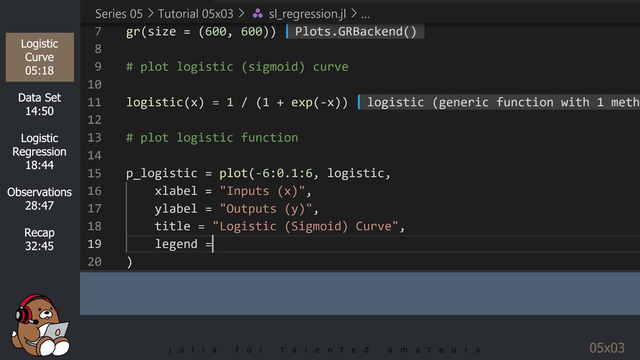 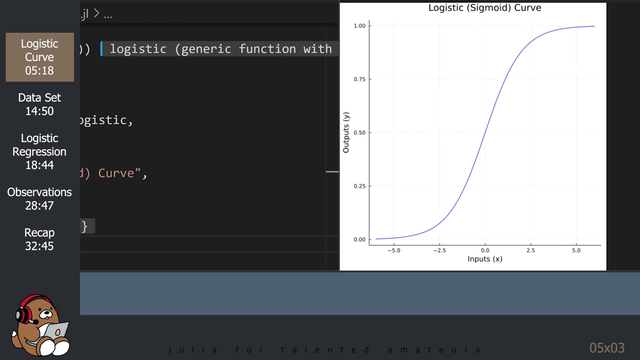 This is essentially a function that allows you to enter Euler's number e to the power of some number. Here we're taking e to the power of negative x. So great, We were able to create our own logistic curve. Now what? 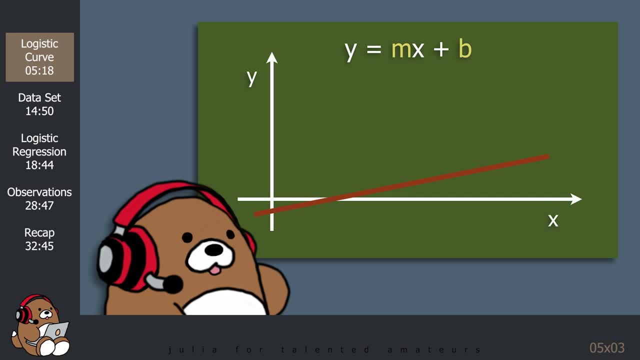 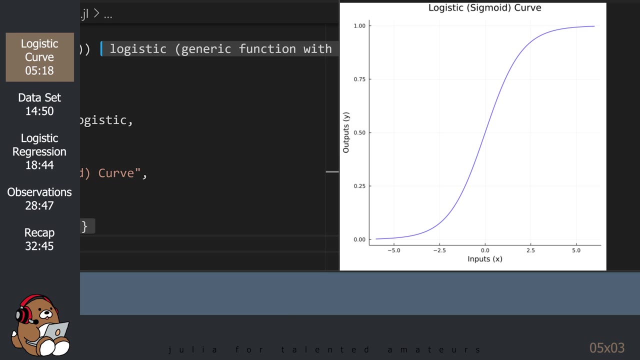 Last week we used the formula for our line y equals mx plus b to find a straight line that was a best fit for our data. We did that by changing the values for the y-intercept and the slope of that line. This week we want to do something similar with the logistic curve. 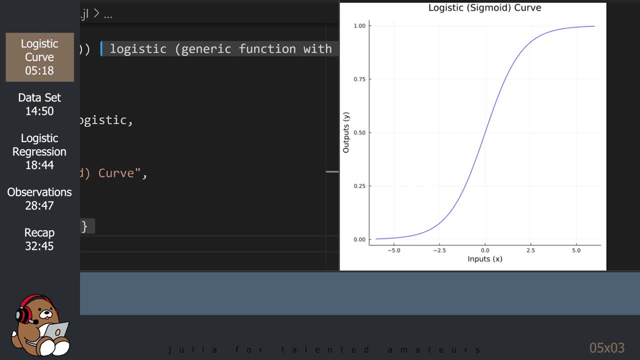 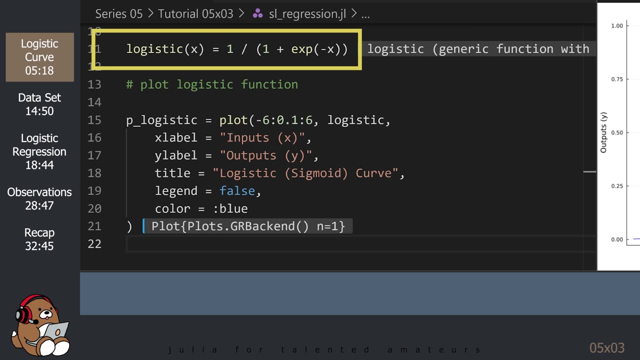 We want to modify the shape of this curve to best fit our data so that we can use it to make classification predictions. But How do we modify this curve? If you look at the formula, there are no parameters or anything like the y-intercept or the slope. 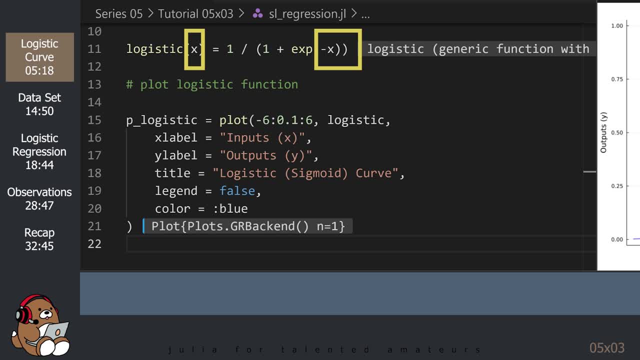 So some clever folks realized that Not only can you enter in a discrete value for x in this equation, you can enter in a function for x, which is what we're going to do. So what function are we going to use? 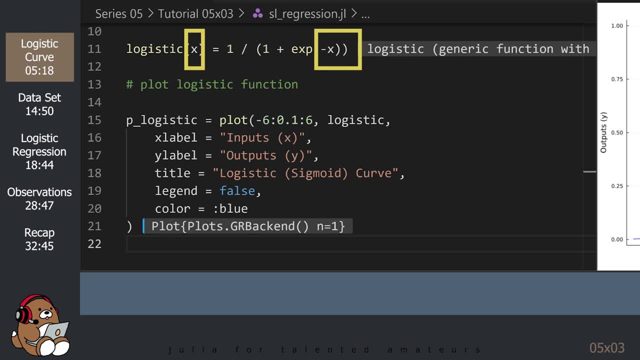 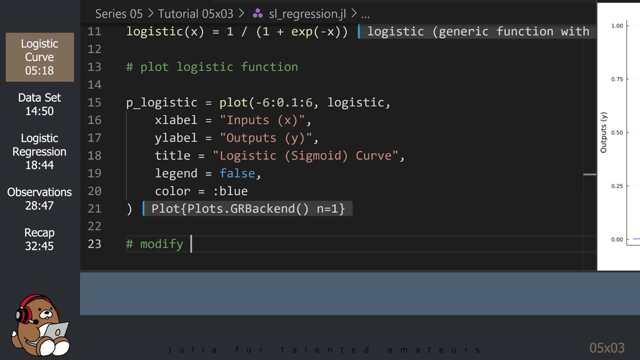 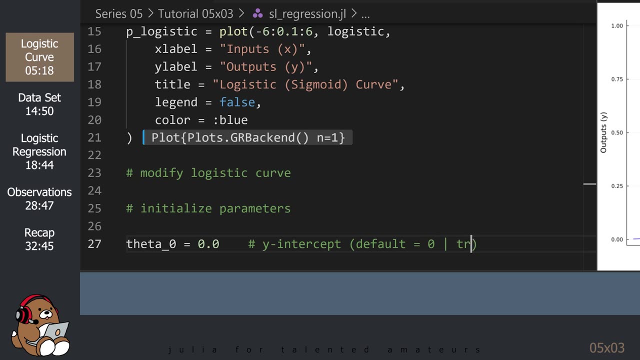 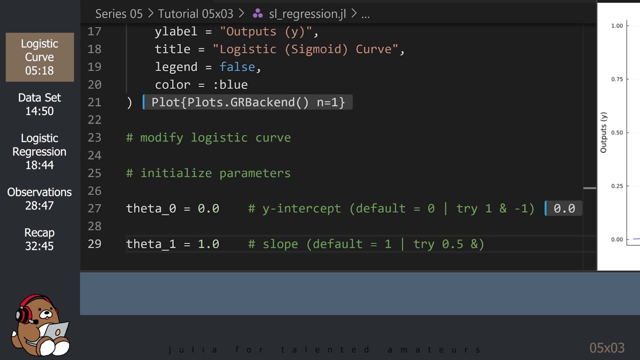 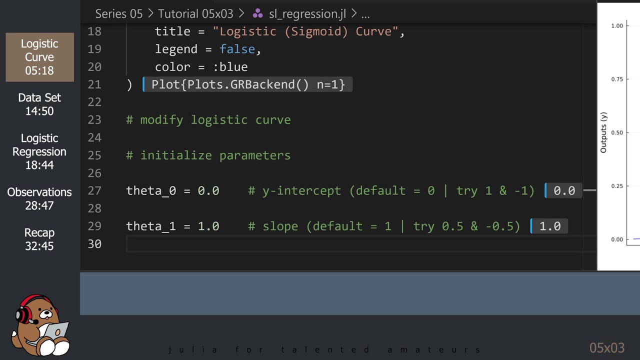 The function that we're going to use is the equation. for a straight line, y equals mx plus b, So we're going to use the equation to work on the y-intercept. These are the same parameters that we used last week For the logistic regression algorithm. Theta 0 is similar in concept to the y-intercept used in linear regression. 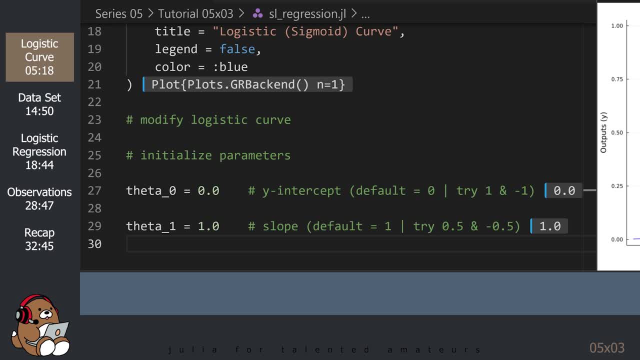 and Theta 1 is similar in concept to the slope used in linear regression, applies both values at 0.. This week I'm setting Theta 0 to 0 and Theta 1 to 1.. These values will generate the default logistic curve that we just plotted. 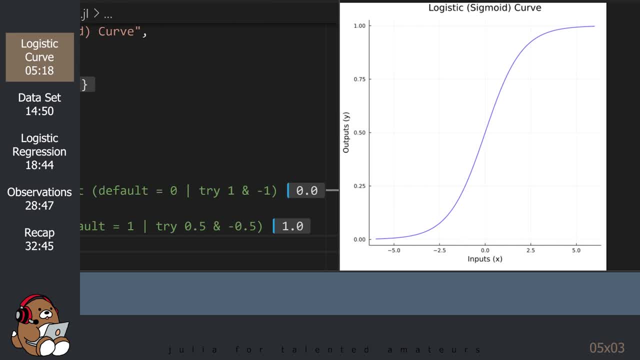 But note that these values do not correspond to the actual Y-intercept or the slope in the default logistic curve. The default logistic curve crosses the Y-axis at 0.5, and there's no equivalent straight line slope, since this is a curve. 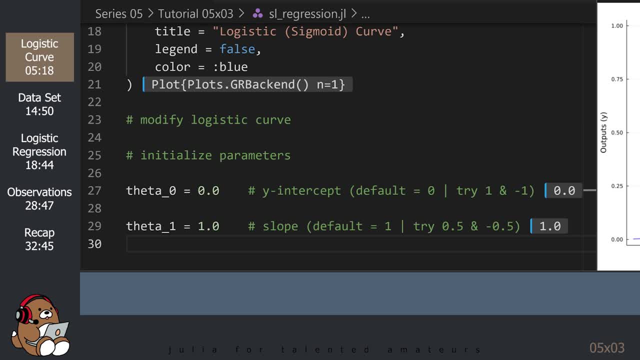 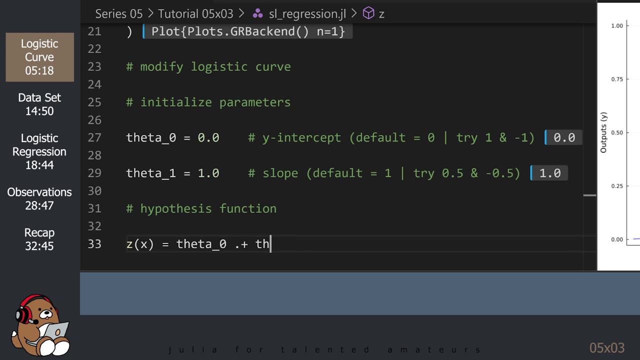 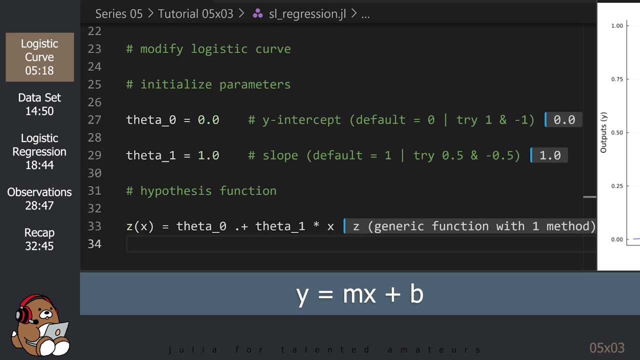 Instead for the logistic regression algorithm, you can think of the parameters Theta 0 and Theta 1 as dials that your computer can turn in order to adjust the shape of the curve. Let's take a look at how to do that. You should recognize this function as the formula for a straight line. Y equals mx plus. 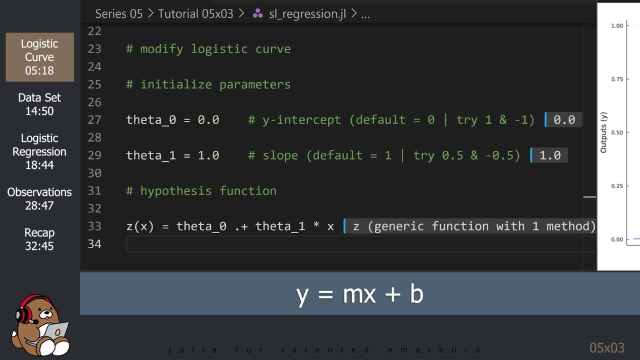 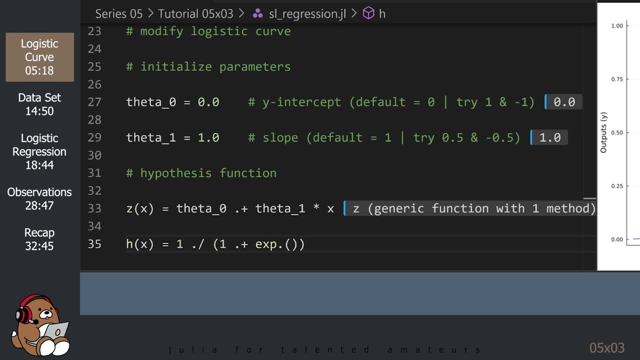 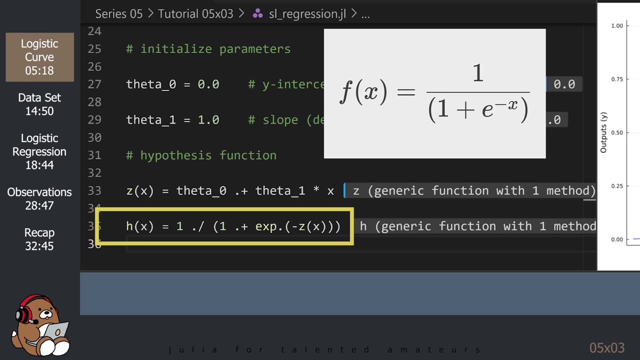 b, which is what we used as the hypothesis function last week. This week we're going to use the logistic curve as our hypothesis function, But we're going to replace the existent equation with a formula for a straight line slope. so 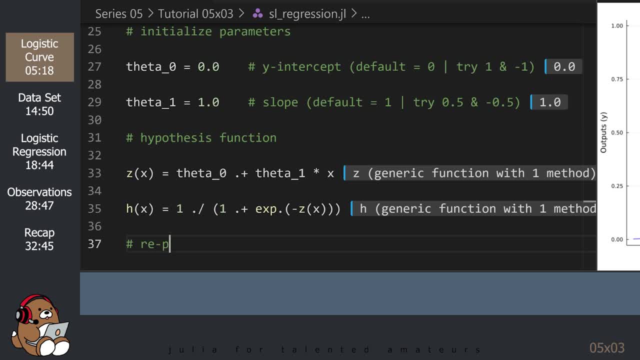 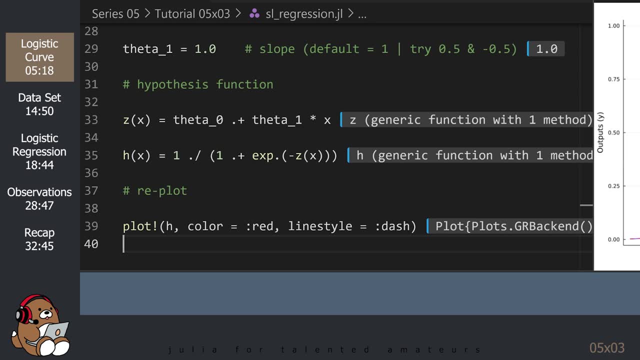 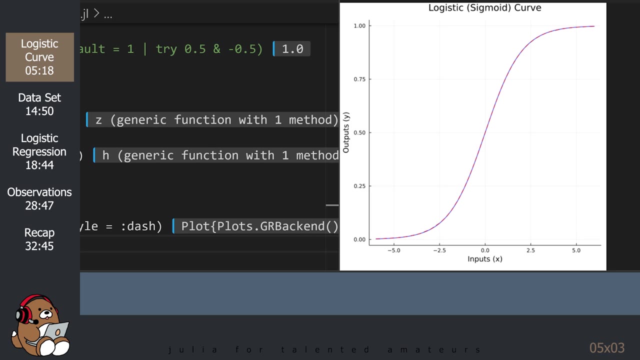 you don't need to worry about that. Anyway, that should do it this time. Thank you for watching line. As you can see, this plot looks exactly the same as the default logistic curve. The difference is that we now have the parameters theta0 and theta1 that we can change in order. 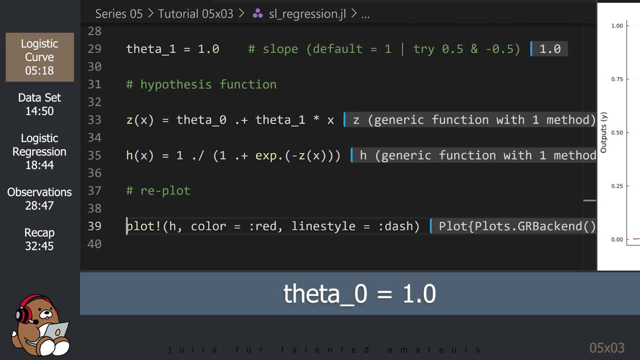 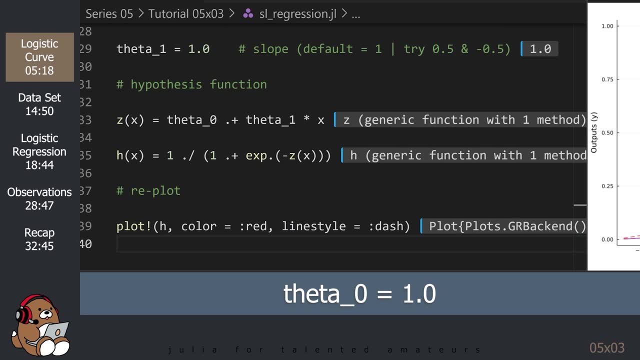 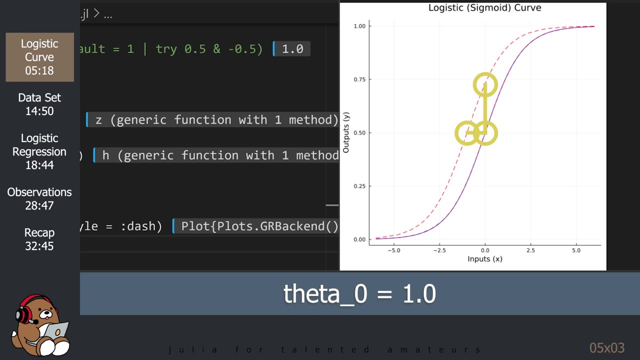 to modify this curve. Change the value of theta0 from 0 to 1 and see what happens. Increasing the value of theta0 moves the y-intercept up along the y-axis. Since the values along the y-axis must follow between 0 and 1, the entire curve does not. 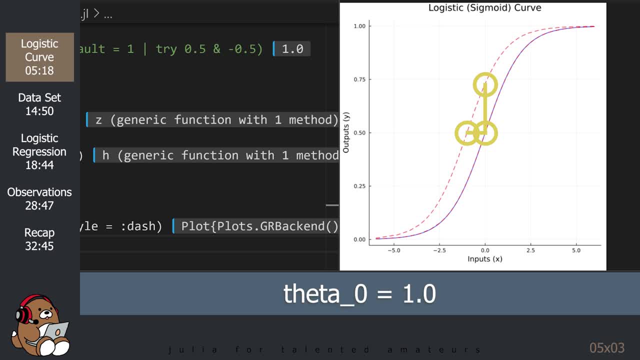 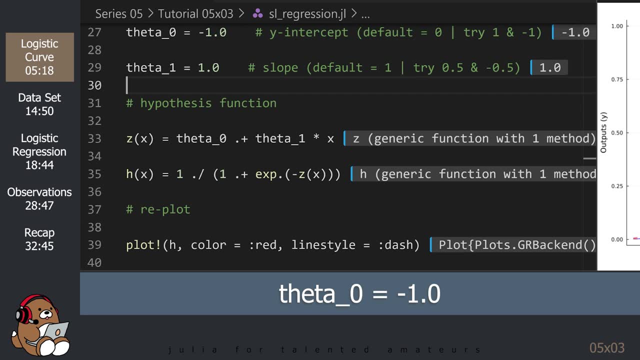 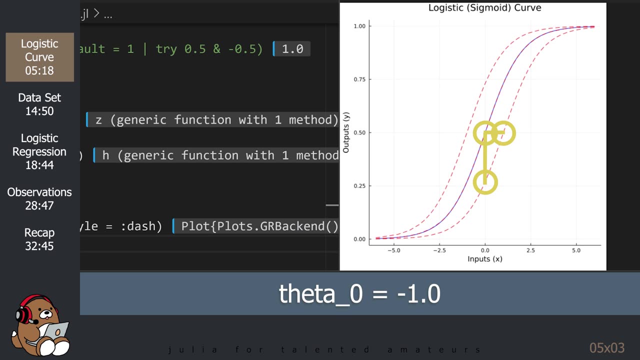 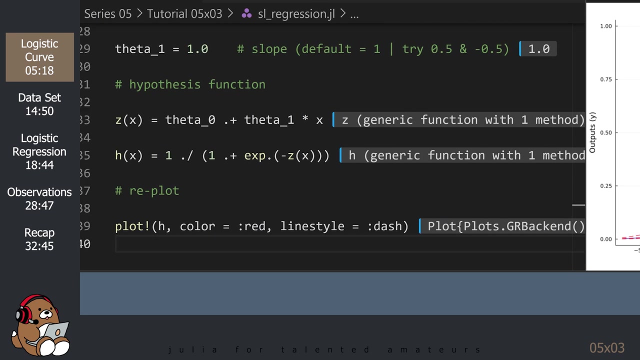 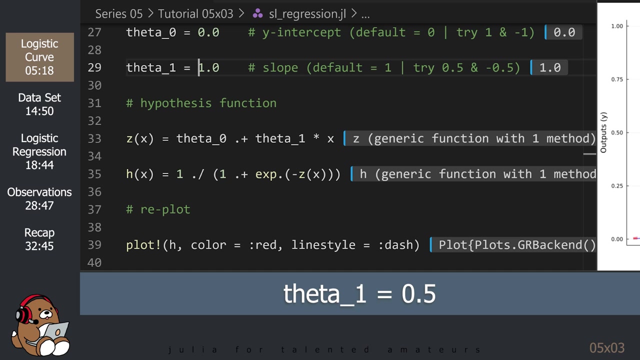 shift up. Instead, the curve shifts to the left. Try changing the value of theta0 to negative 1. Decreasing the value of theta0 moves the y-intercept down along the y-axis, thus shifting the curve to the right. Change the value of theta0 back to 0 and then try changing the value of theta1 from 1 to. 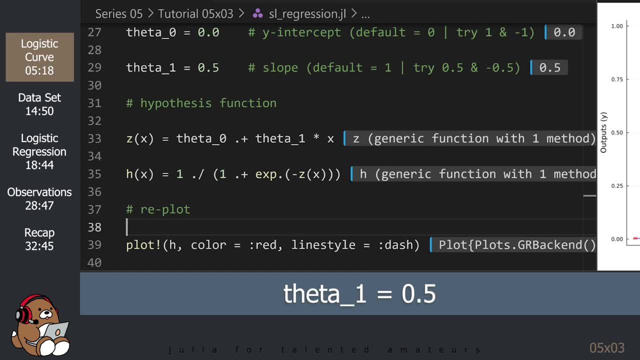 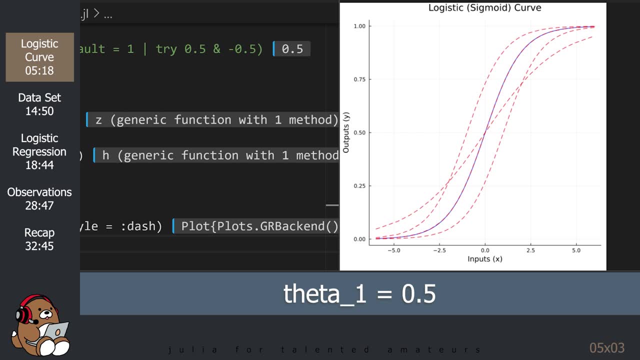 0.5.. Decreasing the value of theta1 from 1 to 0.5.. Decreasing the value of theta1 decreases the quote-unquote slope of the curve, so it makes it flatter as the curve transitions from 0 to 1.. 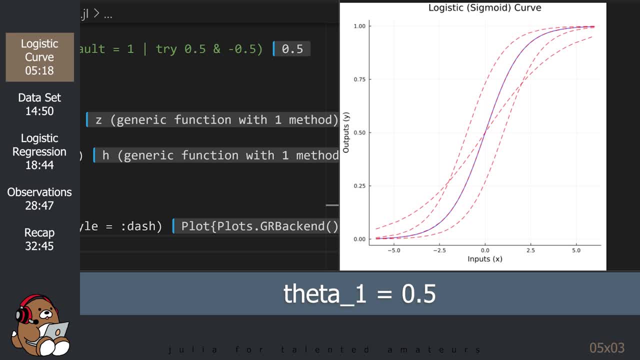 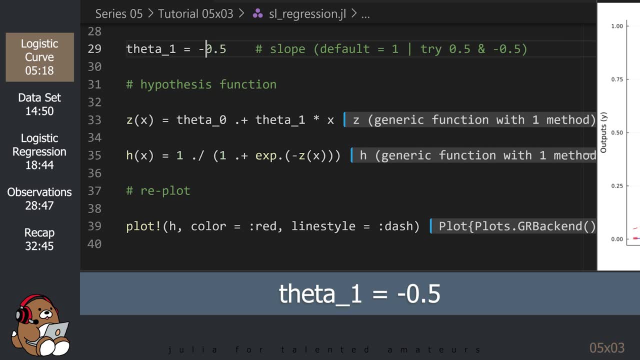 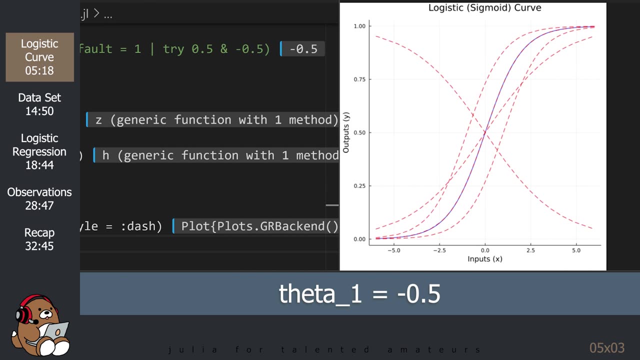 Of course it's not really the slope, but you can think of it that way, since it behaves the same way. Now try changing the value of theta1 from 0.5 to negative 0.5.. Changing a negative value of theta1 results in a downward sloping curve, just like it. 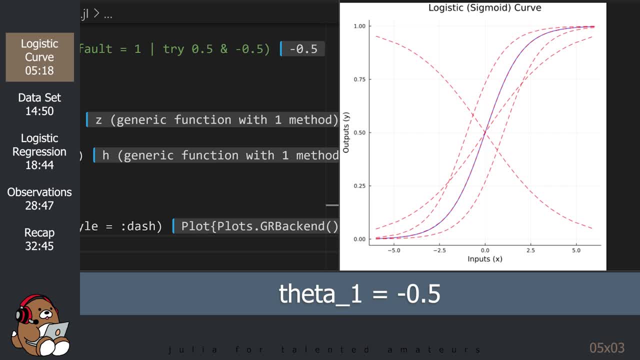 would with a straight line. Pretty cool, right. Go ahead and play around with the settings until you get a feel for how changing the values of theta0 and theta1 will modify the curve. Now that we have a curve that we can modify, let's take a look at our data. 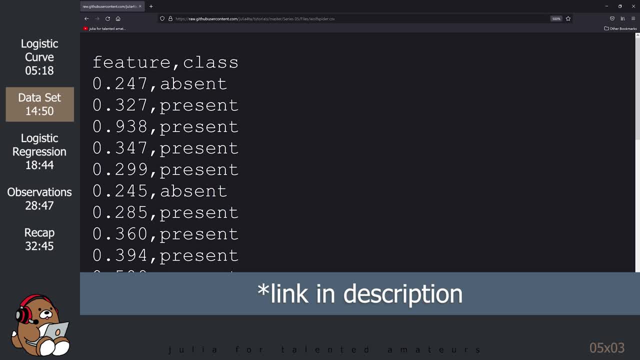 For this tutorial, you will need a data set that will allow you to change the values of theta0 and theta1.. This is a data set that you can download from my GitHub repository. There's a link to it in the description below. You can save it by right-clicking on it. 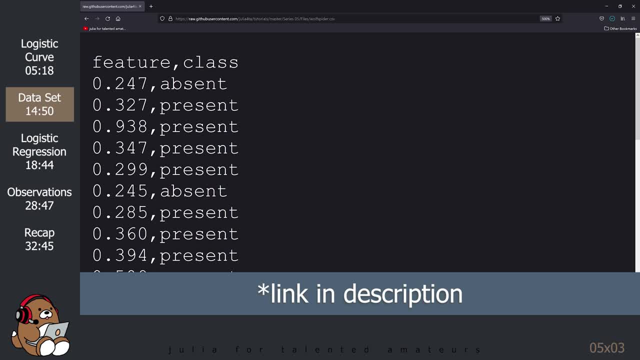 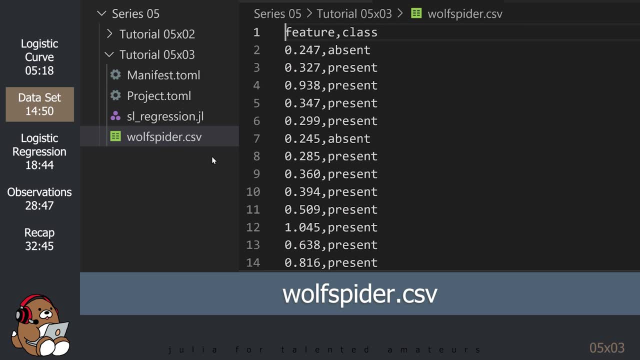 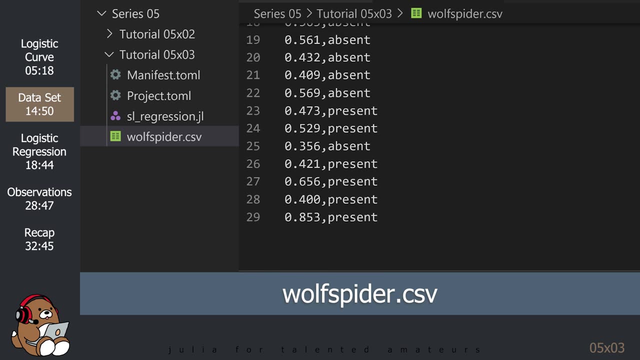 When you download the file, save it to your tutorial directory. It's a CSV file called wolfspidercsv and it contains a collection of input-output pairs showing the size of grains of sand as the input or feature and showing a binding value. 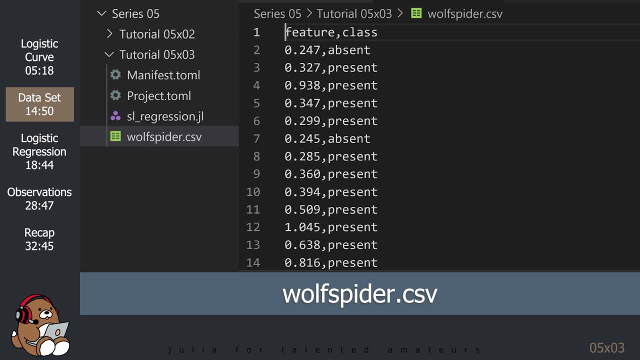 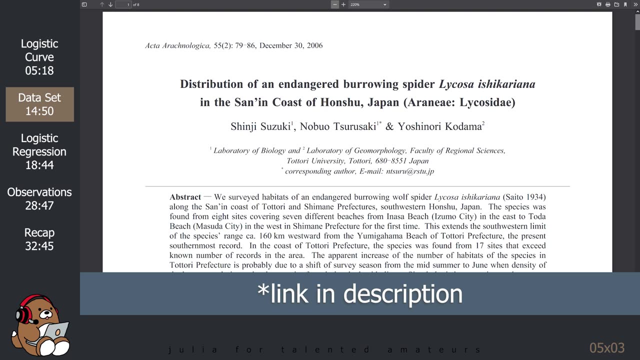 binary output as either present or absent, indicating either a positive or negative class testing for the presence of a wolf spider in the sands. This data is from a 2006 research paper by Suzuki, Tsurusaki and Kodama titled Distribution. 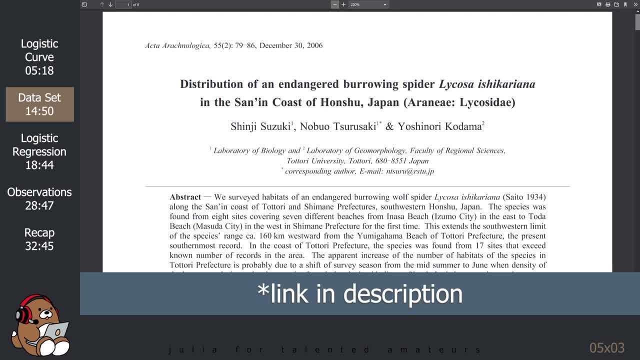 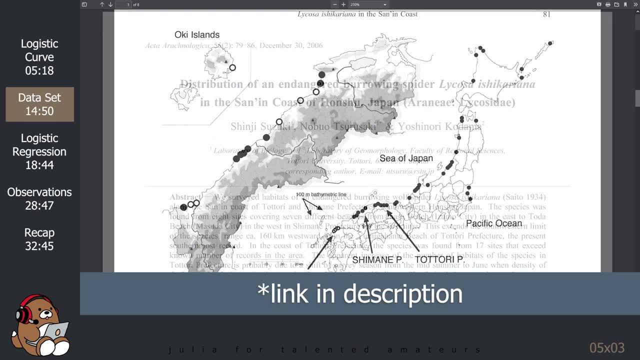 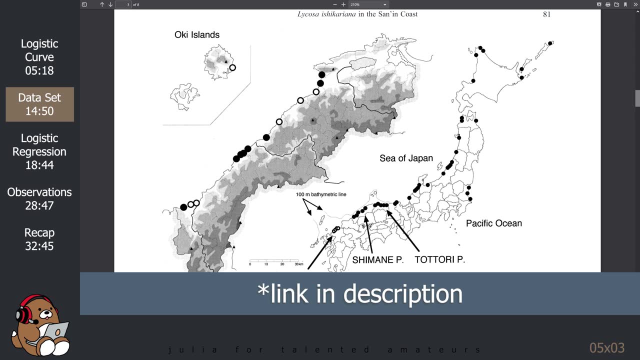 of an Endangered Burrowing Spider in the San'in Coast of Honshu, Japan. I apologize for my pronunciation. In the interest of conservation, the researchers surveyed habitats along various beaches in Japan, where they were looking for the presence of an endangered burrowing spider. commonly, 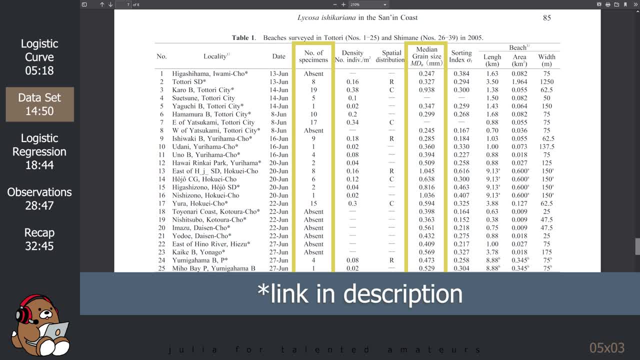 known as the wolf spider. We're going to use a simplified version of the data presented in their article as our motivating example in order to build a logistic regression model that we can use to predict the probability of the presence of wolf spiders, based solely on the size of grains of sand. 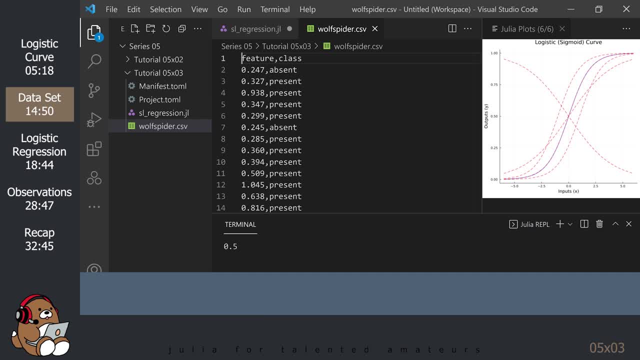 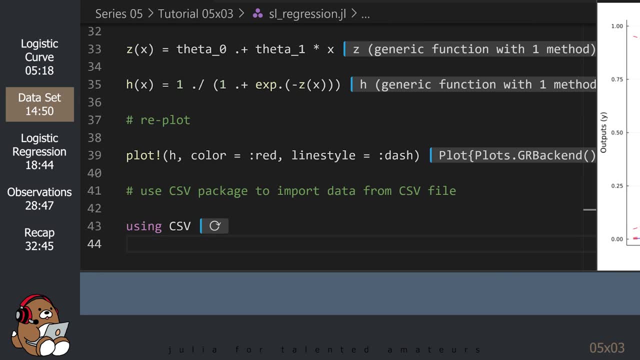 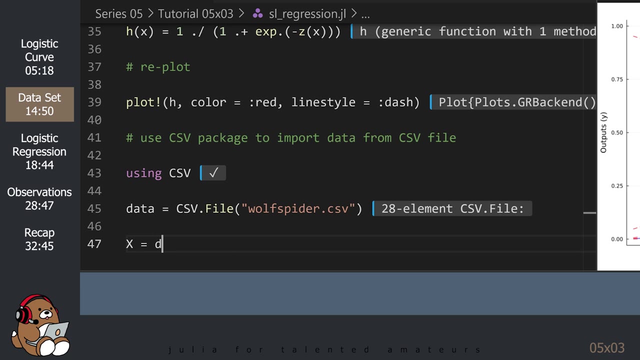 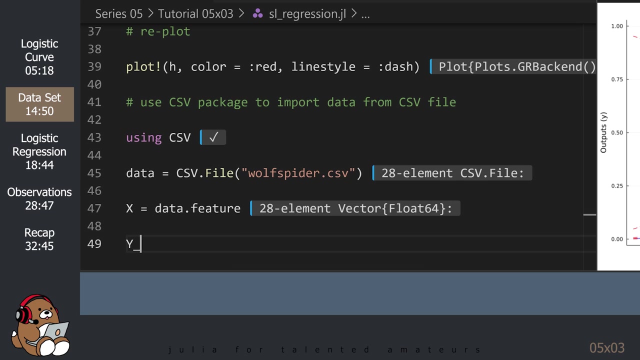 or the size of sand on a beach in Japan. Now that we have our data stored on disk, let's load it into memory. This is the input data that measures the grain of sand in millimeters. This is the output data, which is a string that is either present or absent. 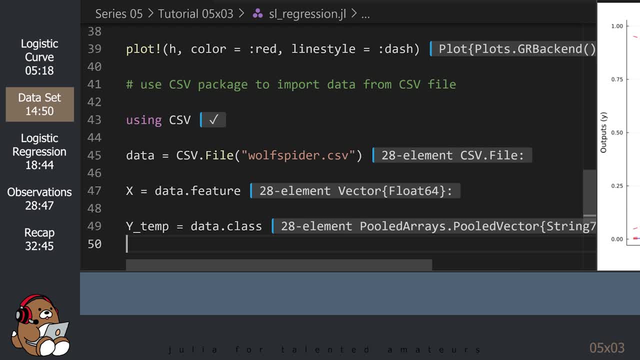 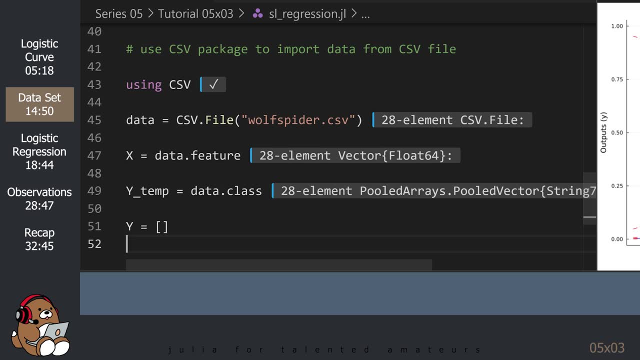 The output data measures the grains of sand in millimeters. The output data will print an output of a string that is either present or absent for a positive class, or Absent for a negative class. In order for us to use this data, we need to convert the Strings into either a: 1 for. 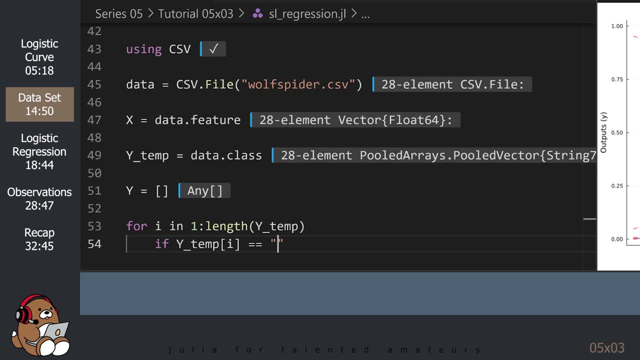 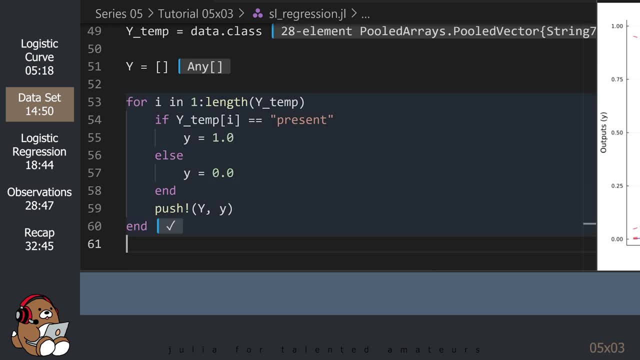 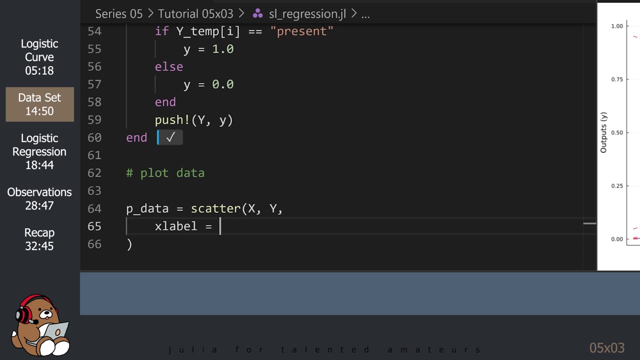 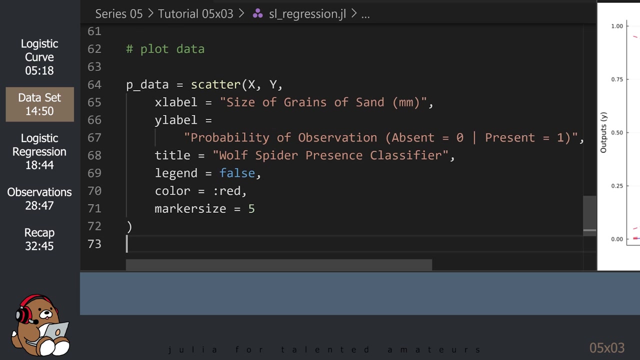 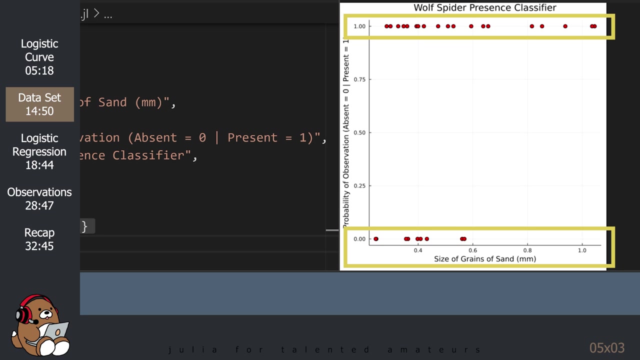 a positive class or a 0 for a negative class. OK, now that we have our data loaded into memory, let's plot it and take a look at it. As you can see, all of the data points are either 0 or 1 along the Y-axis. 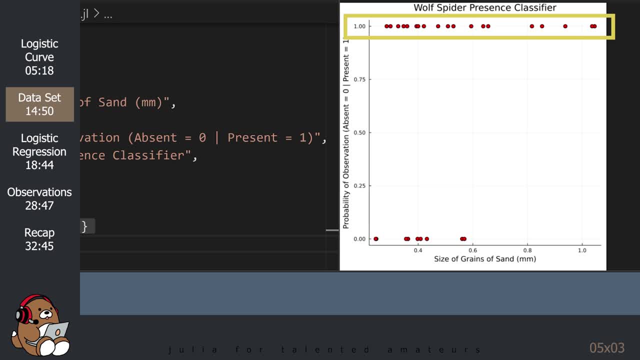 Interestingly, the Wolf Spider seems to be present regardless of the size of the grains of sand, but it's only Absent when the grains are relatively small. Just by looking at this data, it's not obvious how you might use the size of the grains of. 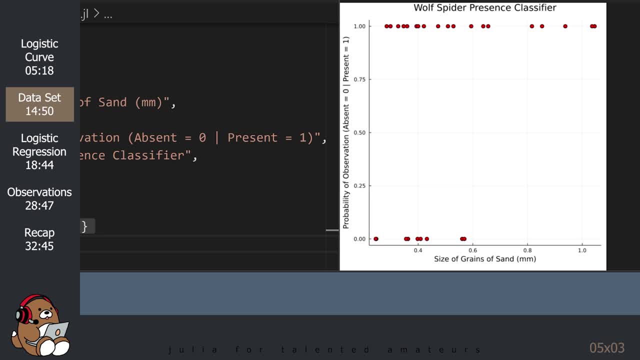 sand in order to predict the Presence or Absent size. Instead, what we want to do is to fit a logistic curve to this data in order to generate a model that we can use to predict the Probability of the Presence of the Spider, given the grain. 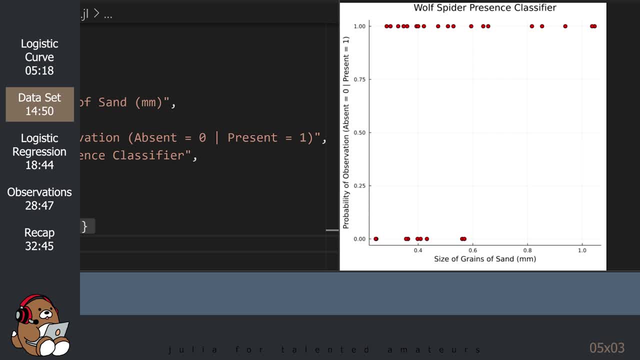 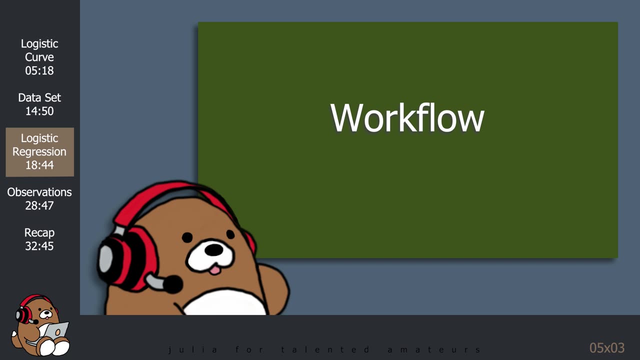 size. Again, just by looking at the data, it's not obvious how to find a best-fit logistic curve for this data. That's why we need Machine Learning, Even though we're trying to solve a Classification problem rather than a Regression problem, we're 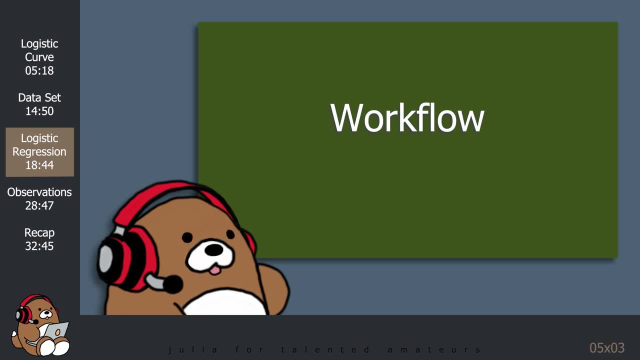 going to follow the exact same Machine Learning workflow that we used last week. As a reminder that workflow includes these steps: 1. Initialize the parameters. 2. Define a Hypothesis Function. 3. Define a Cost Function. 4. 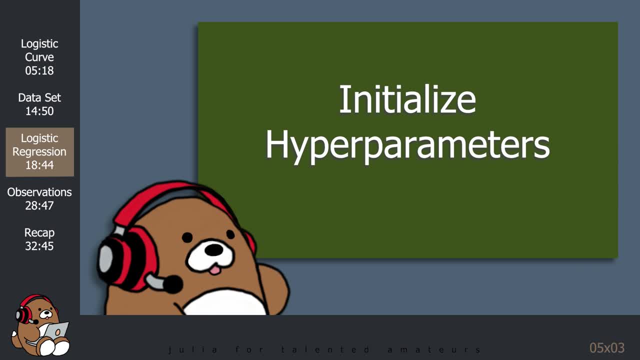 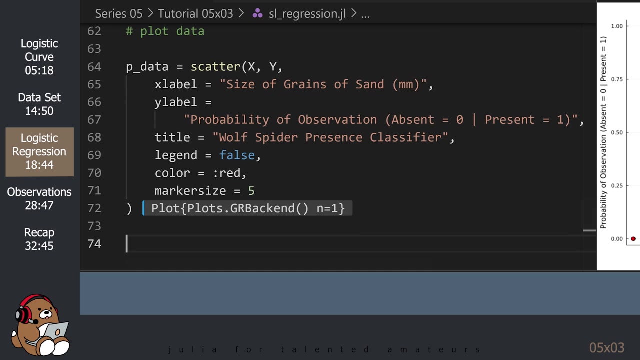 Define an Optimization Algorithm, 5. Initialize the Hyperparameters, 6. Change the Values of the Parameters, 7. Recalculate the Cost, 8. Iterate until an optimal value is found for the Cost. While the overall workflow is the same, the actual functions that we will be using will: 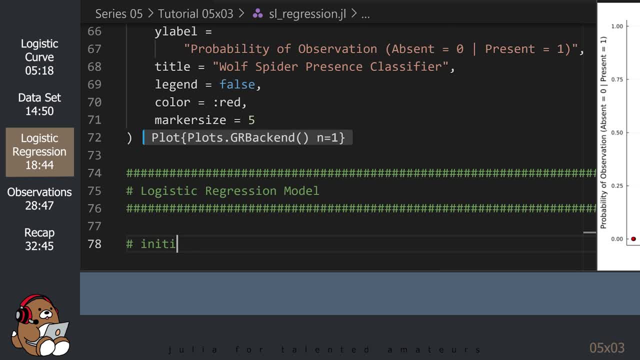 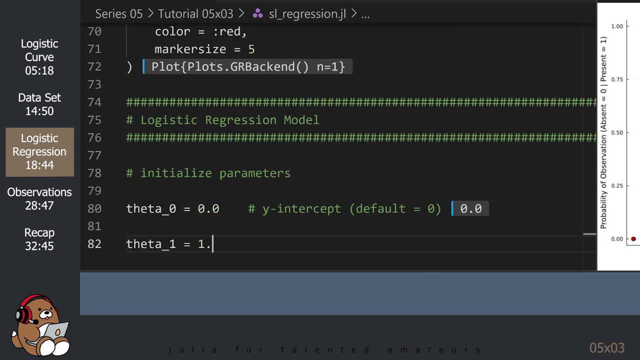 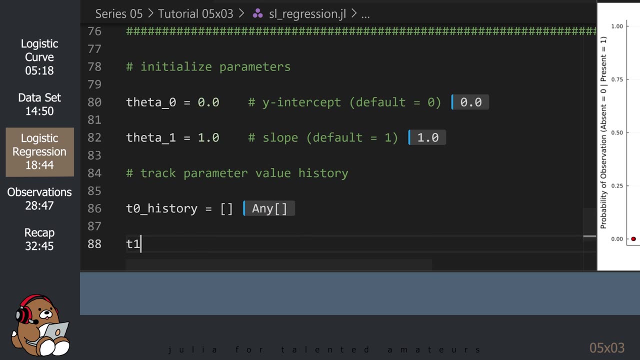 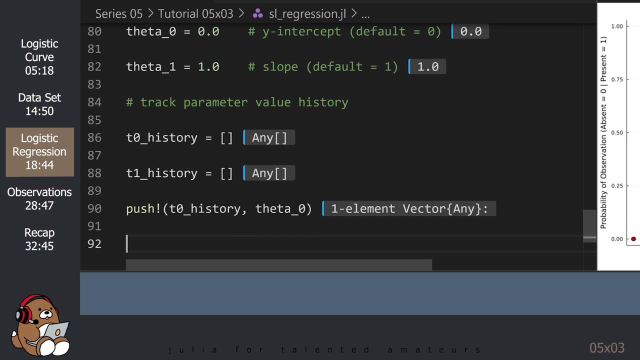 be slightly different. Let's start by initializing the parameters This week. let's track the values of both Theta0 and Theta1 so that we can see how they change over time. Next, we need to define our Hypothesis Function. Next, we need to define our Hypothesis Function. 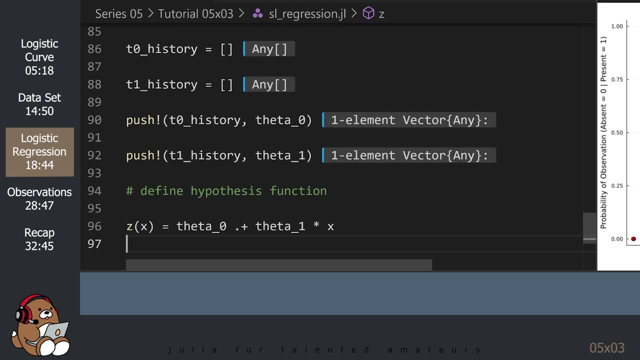 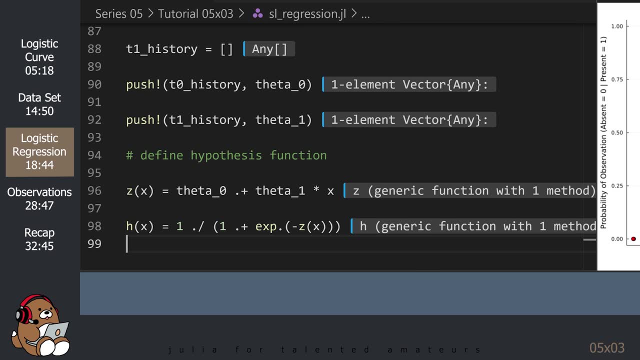 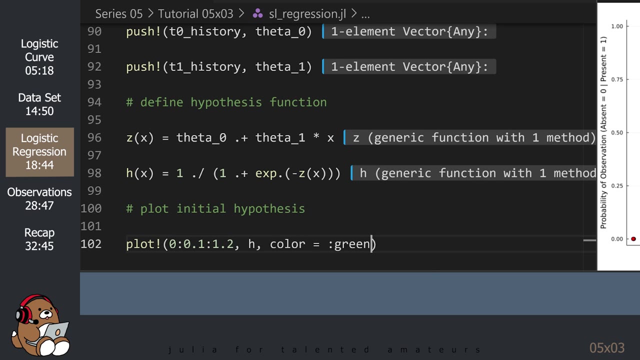 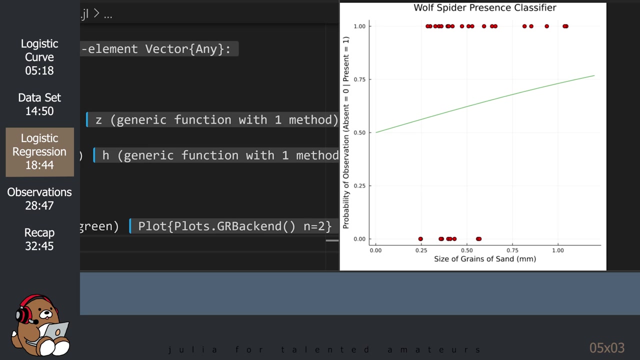 Next, we need to define our Hypothesis Function. Let's add this Initial Logistic Curve to our plot. Let's add this Initial Logistic Curve to our plot. So this green curve is the Initial Logistic Curve. The reason why it doesn't look like the S-shaped curve that we saw earlier is because we're 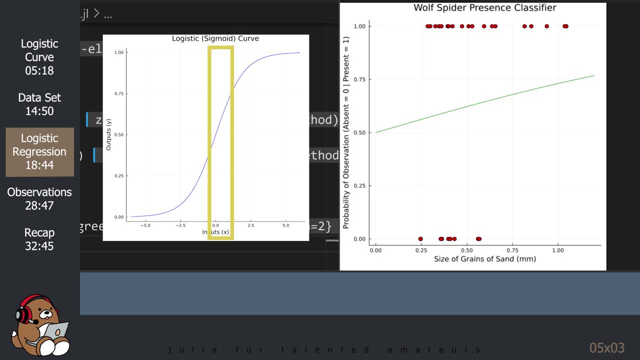 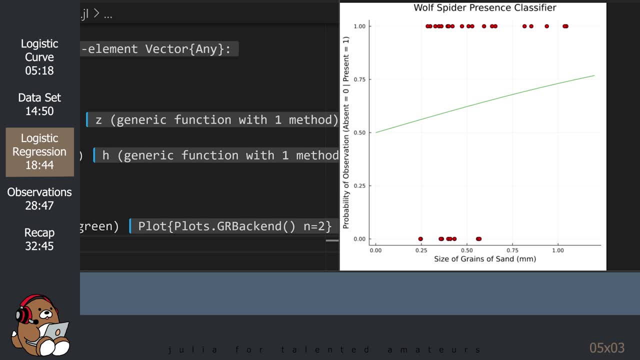 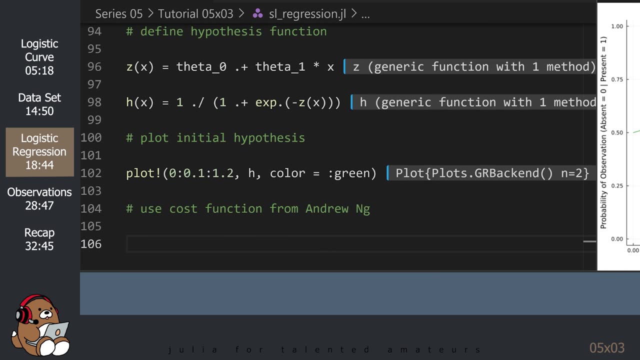 only seeing the range when x is between 0 and 1.. Somehow we need to get our computer to learn how to modify this curve so that it does a better job of fitting our data. In order to do that, we need to define a Cost Function. 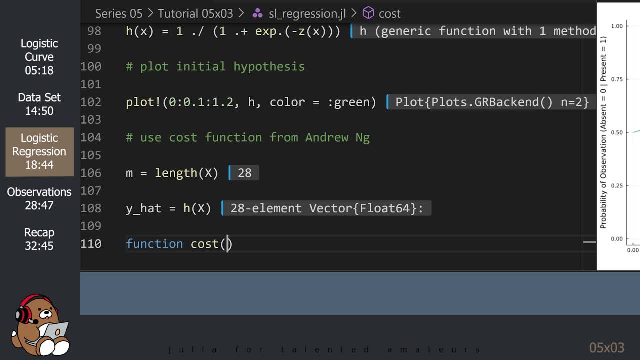 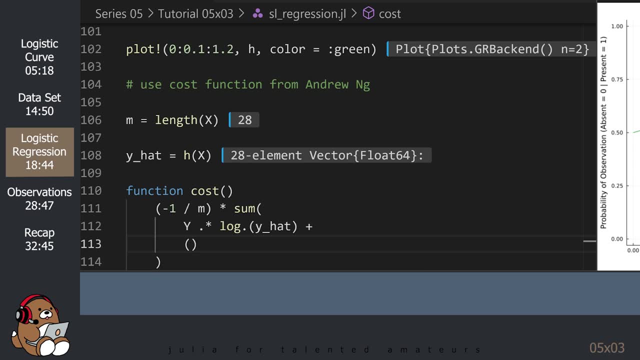 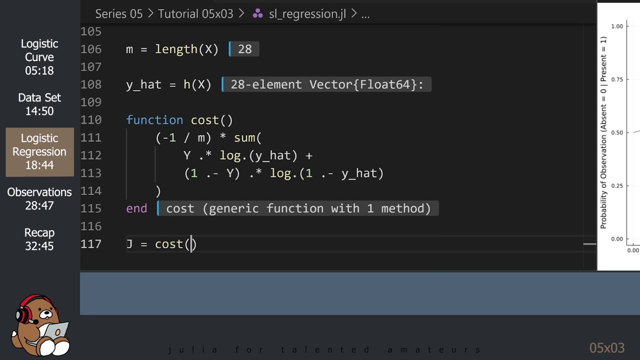 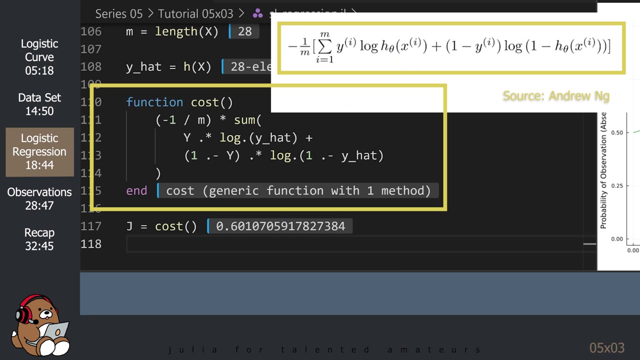 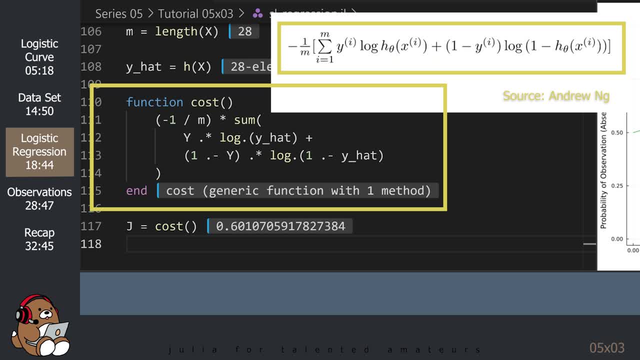 It looks really scary, since it has the Log Function in it. Just like last week, I'm using the equations from Andrew Ng. Without getting into the math, here's how you can think about this cost function. When defining any cost function in machine learning, you want a function that rewards. 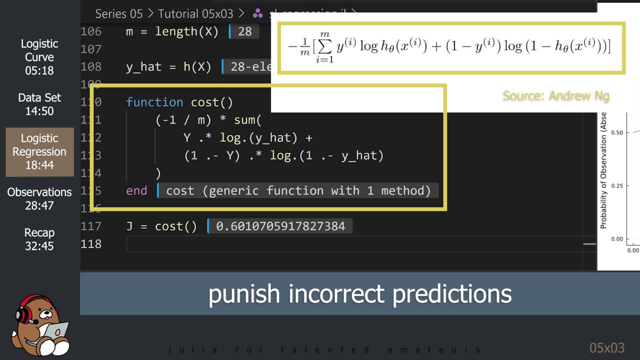 correct predictions and punishes incorrect predictions With this cost function. if your computer predicts a class of 1 when the actual class in the dataset is 0, then your computer will pay a large penalty, meaning that the cost will be high. Conversely, if your computer predicts a class of 1 and the actual class in the dataset is, 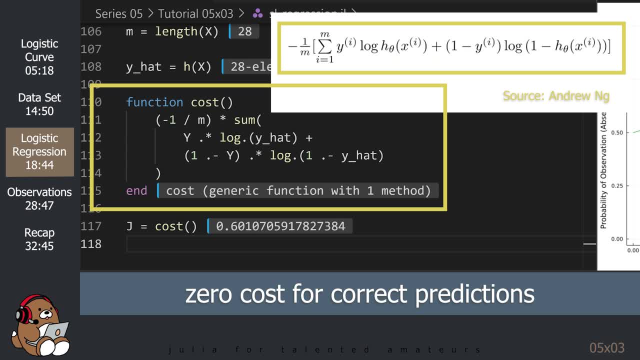 1,, then your computer will not pay a penalty at all, meaning that the cost will be 0. Based on how this function is designed, all your computer needs to do is to adjust the parameters until it finds a minimum value for this cost function. 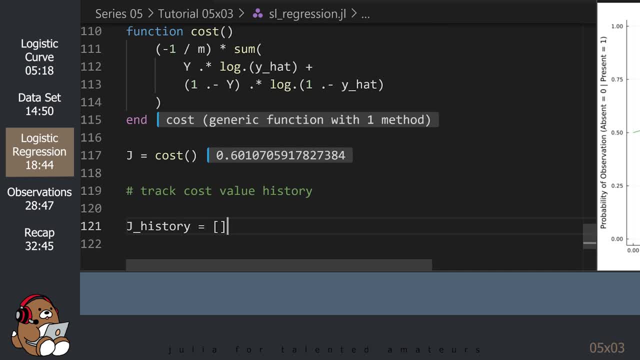 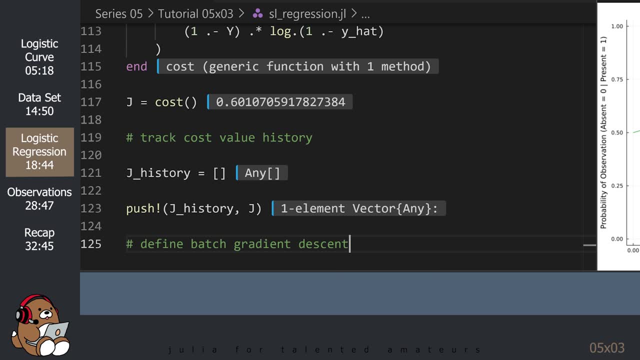 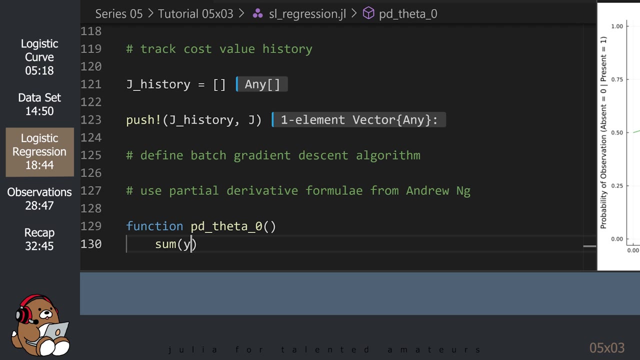 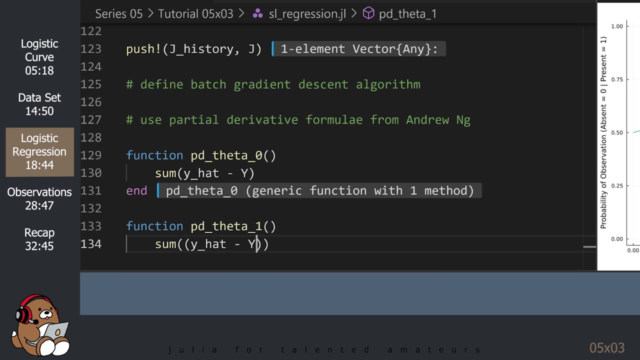 Just like we did last week, let's keep track of this cost over time. Next, we need to define our optimization algorithm. Just like we did last week, we'll be using the Batch Gradient Descent algorithm, But because our cost function is different, the partial derivative function will also. 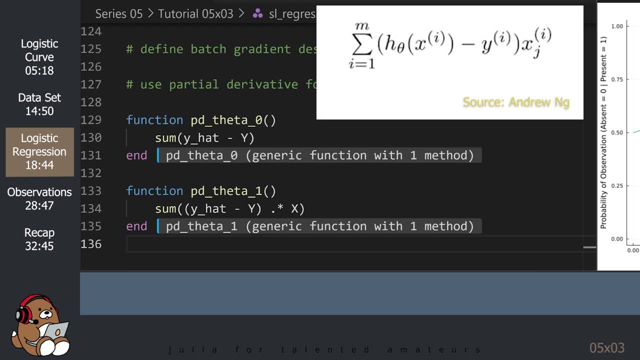 be different. These functions are the result of taking the partial derivatives of the cost function, As we discussed last week. these functions will calculate the direction and the magnitude of the changes that your computer will need to make to the parameters in order to lower the value of the cost function. 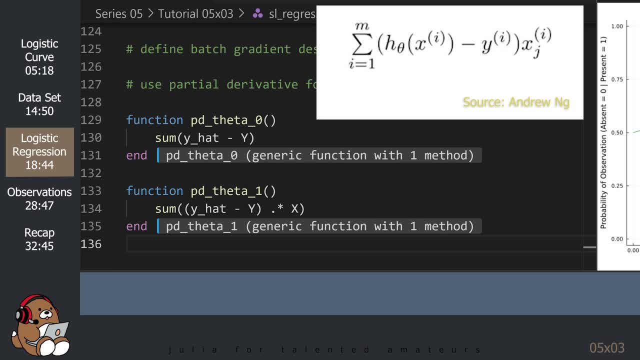 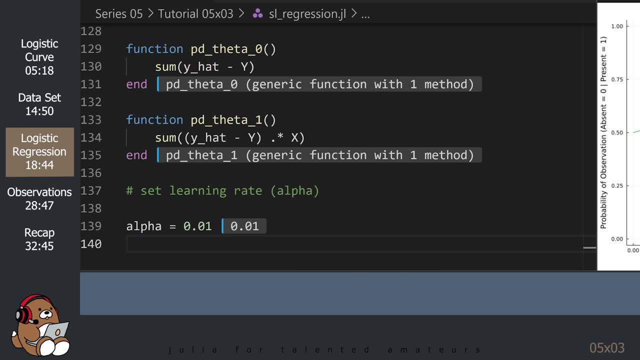 Once again, these equations are from Andrew Ng. Next, let's initialize our hyperparameters. Unlike last week, when I cheated when setting the learning rates, this function will be set to 0.01.. This week, I'm using the default learning rate of 0.01 for all parameters. 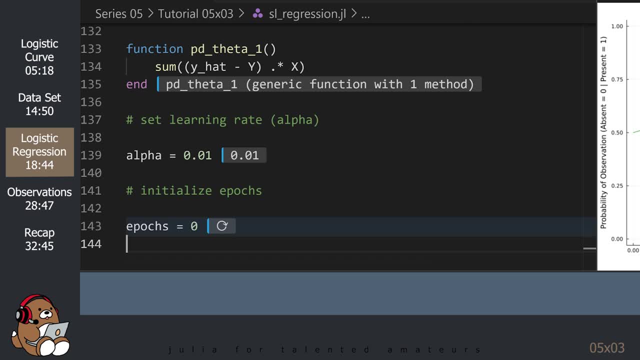 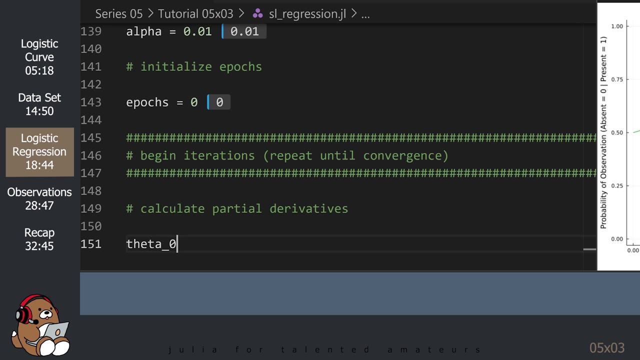 Last week we did everything manually, so we didn't have that many epochs. But this week we're going to go through many iterations, so this number will be more significant. Next we need to set up the steps needed for our iteration. 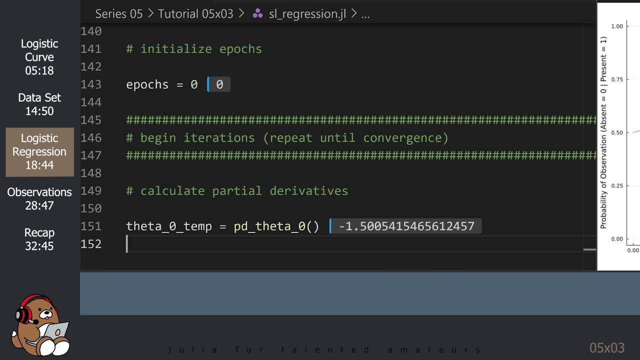 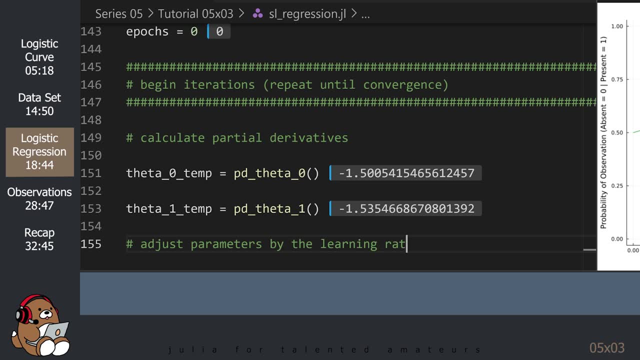 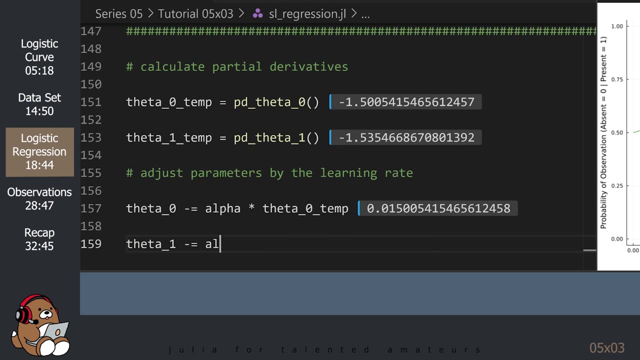 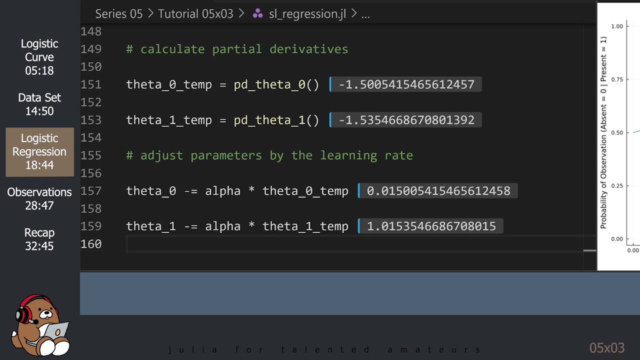 These steps are nearly identical to the steps that we used last week, So let's pause here and take a look at the numbers. The value of theta0 increased from 0 to 0.015,, meaning that the y-intercept shifted only. 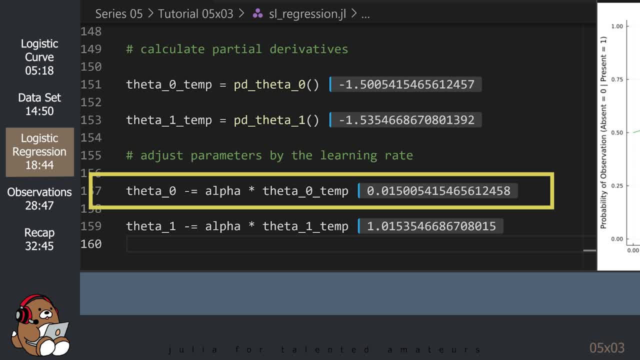 up slightly, which caused the curve to shift slightly to the left. The value of theta1 increased from 1 to 1.015, meaning that the slope of the curve increased slightly, so that it's slightly steeper as it transitions between 0 and 1.. 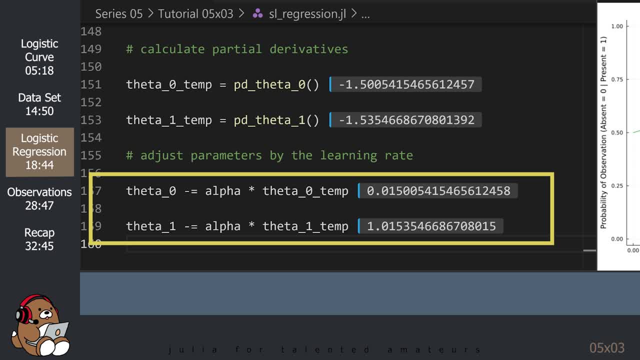 The other thing to note is that, with a learning rate of 0.01, these incremental changes are very small. So we will need to repeat this process. So we will need to repeat this process. So we will need to repeat this process many times. 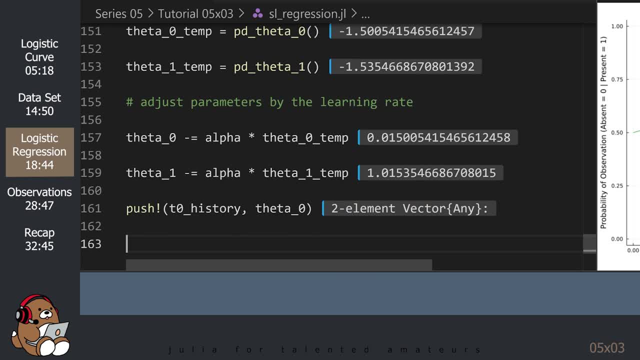 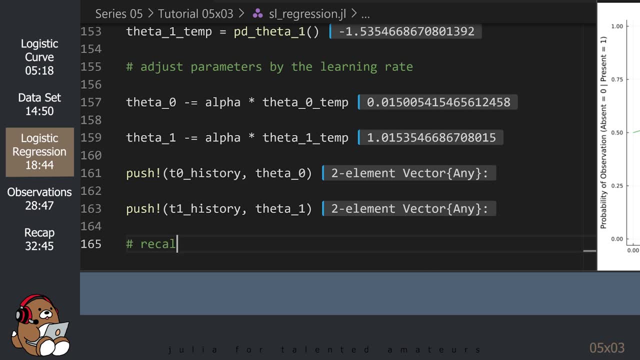 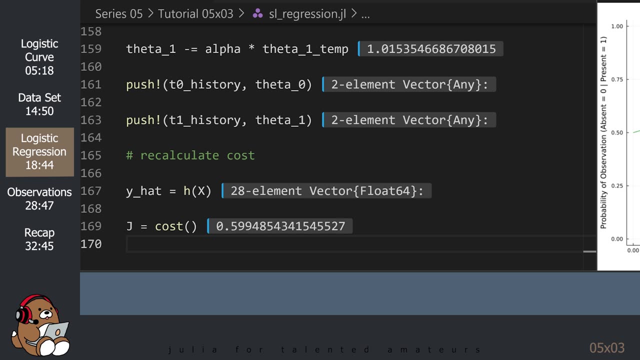 Let's keep track of the values of these parameters And now let's recalculate the cost to see if our cost improved at all. So the value of our cost function decreased from 0.601 to 0.599.. That's not a very big improvement, but it is an improvement. 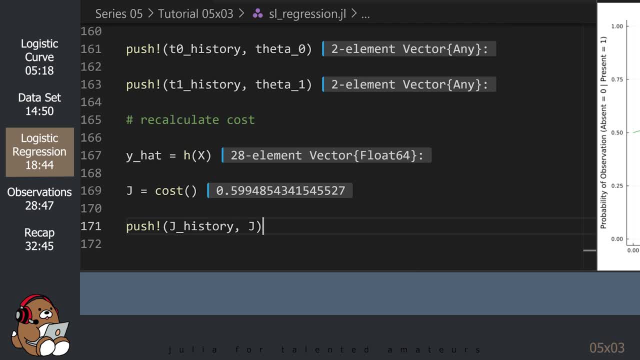 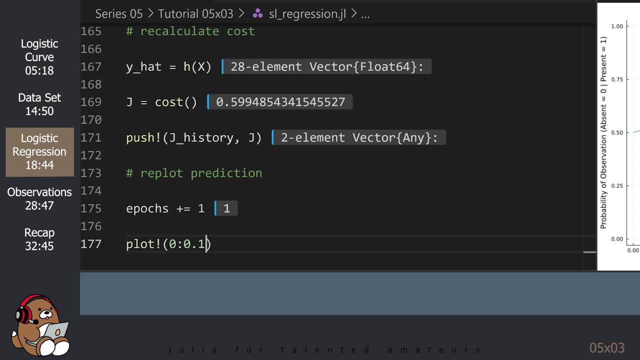 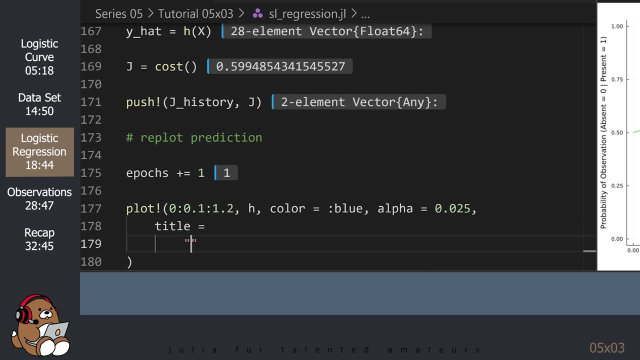 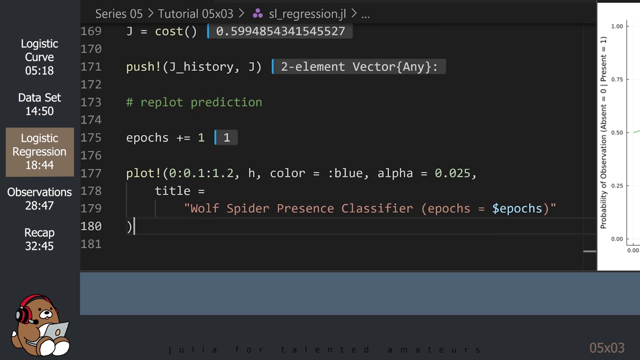 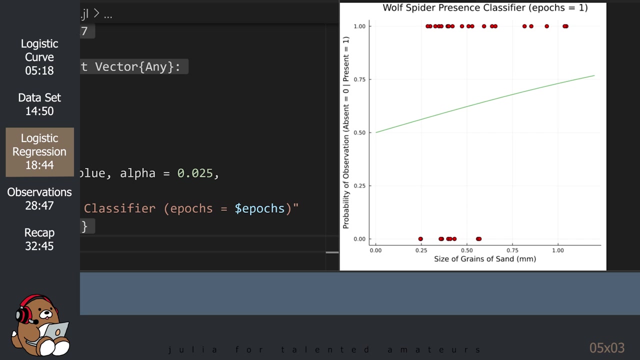 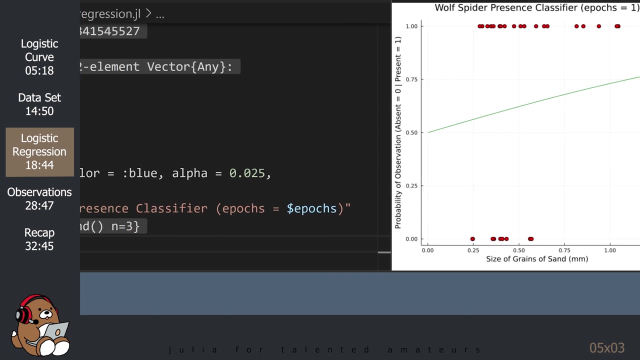 Let's keep track of this value and then add the new curve to our plots. So, other than adding the epochs to the title, it doesn't look like anything has changed on this plot. Unfortunately, the change is too small to be noticeable. 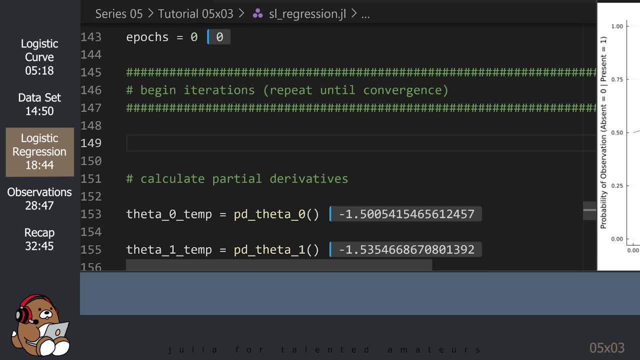 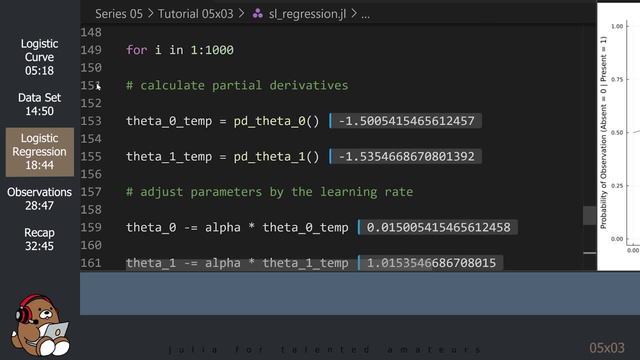 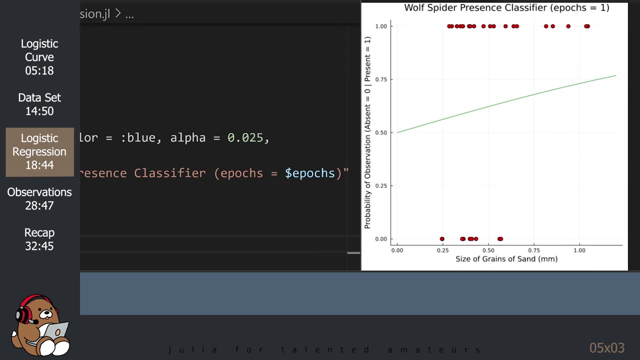 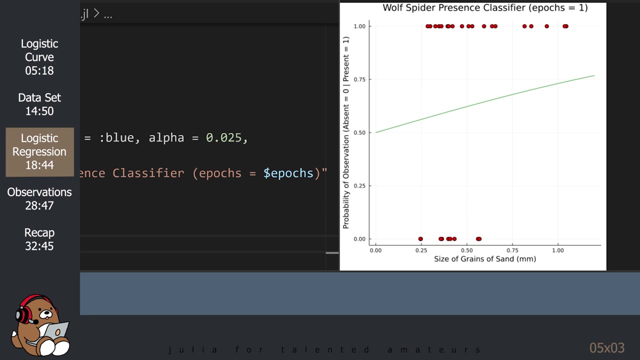 Let's set up a for loop so that we can iterate this process 1,000 times. So what happened? There are no outputs in the REPL and the plot looks the same. Did our for loop do anything? When using the for loop, it looks the same. 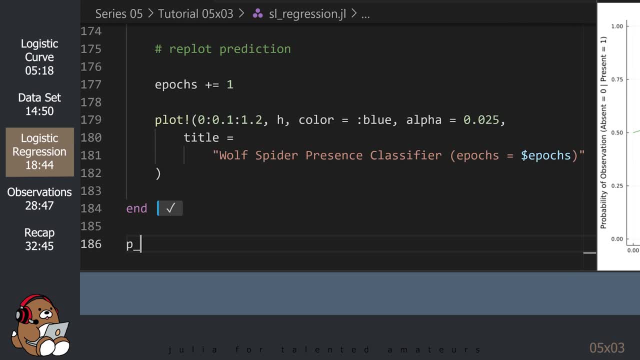 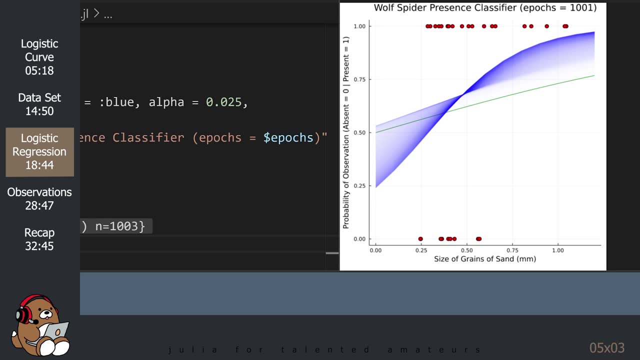 When using the for loop, it looks the same. When using the for loop, it looks the same. When using the Plots package, you need to call the name of the plot in order to display any updates. Okay, so that looks really interesting. 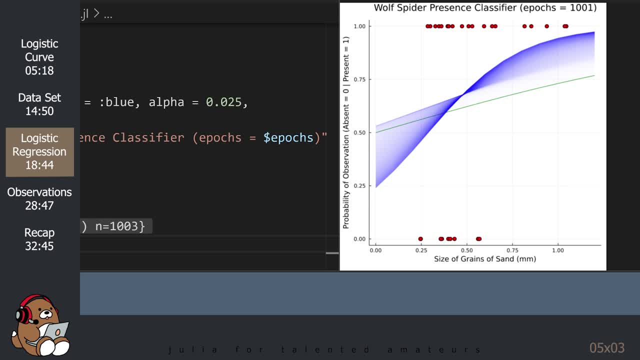 What's going on here? The lighter shades of blue indicate the early iterations. The darker shades of blue indicate the most recent iterations. It looks like that initially the y-intercept of the curve moved up, but over time the y-intercept moved down. 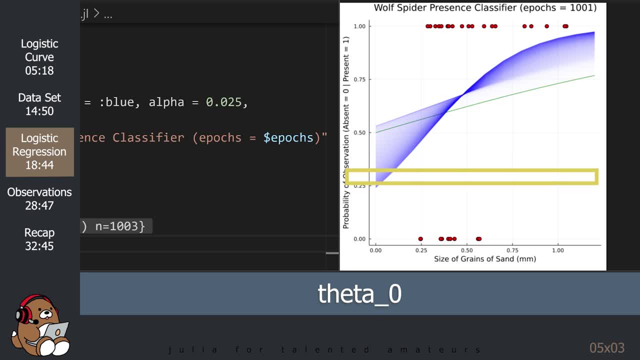 so now the y-intercept is much lower than the y-intercept of the initial green curve. Also, the slope of the curve has continued to increase over time, so now the curve is much steeper than the initial green curve. The curve is starting to look like the logistic curve. 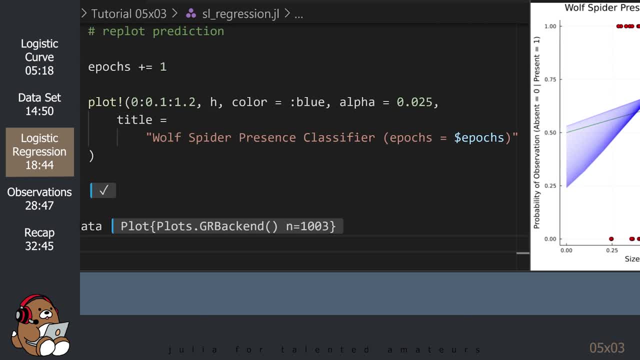 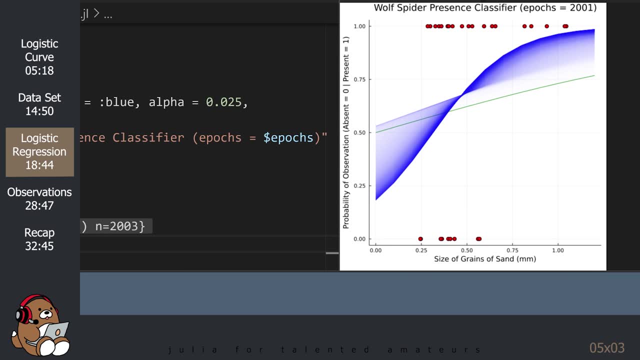 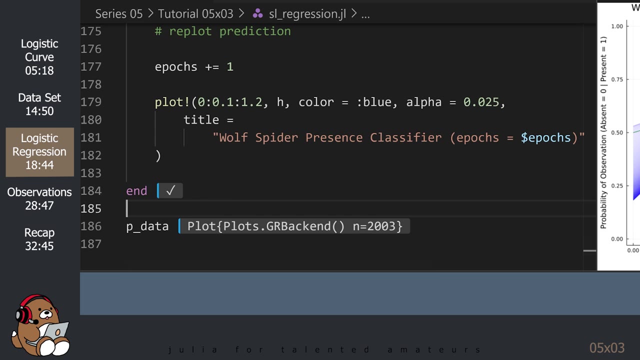 but it still doesn't seem to fit all of the data, so let's run this iteration 1,000 more times. It looks like there's been some improvements, but the improvements are definitely starting to slow down. Let's run it 1,000 more times to see if that does anything. 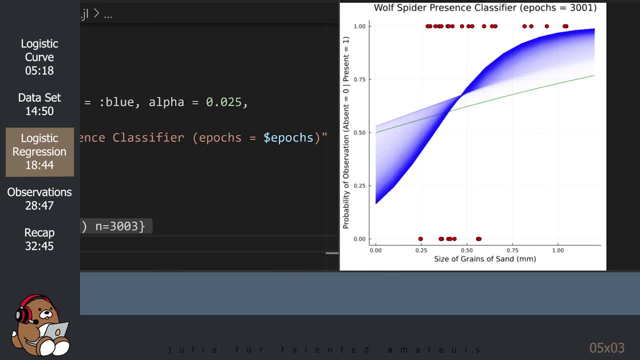 It looks like there's a slight improvement, but it's becoming harder to see. Let's run it 1,000 more times until we get to 4,000 more times. Let's run it 1,000 more times until we get to 4,000 epochs. 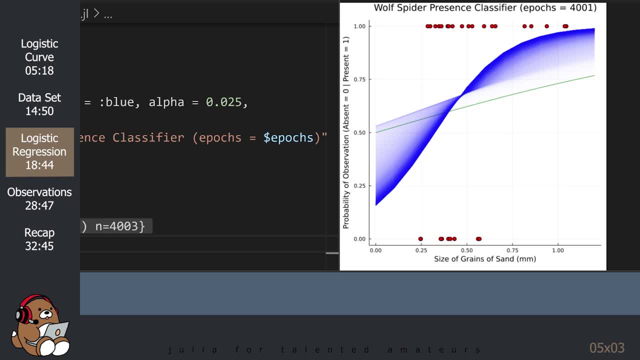 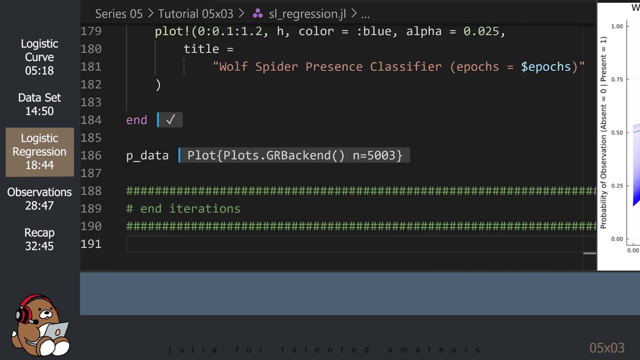 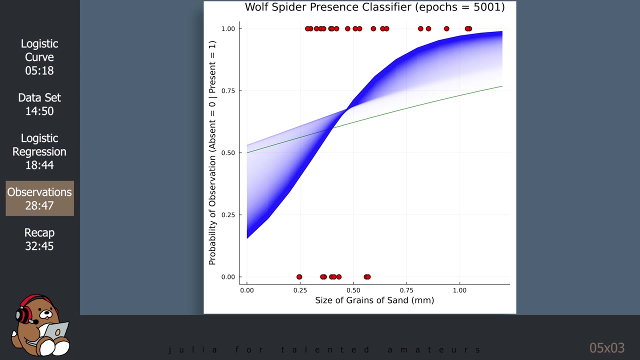 Yeah, it's definitely slowing down. Let's run it 1 more time, Okay, so this time the difference is barely noticeable, so let's stop here and talk about this plot. So the way to read this plot is that the darkest blue line. 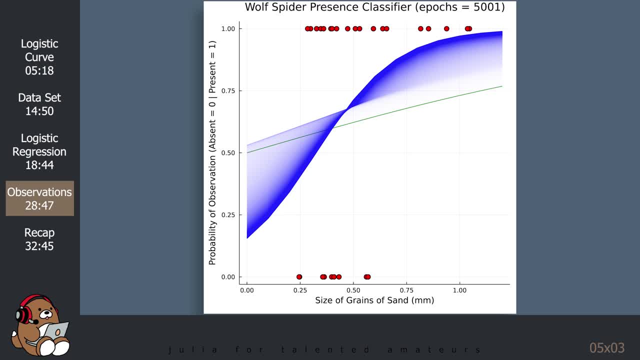 is the model that best predicts the presence of a wolf spider, based on the size of the grains of sand on the beach. So the larger the grain size, the higher the probability, and the smaller the grain size, the lower the probability. Notice that the probability never gets close to zero. 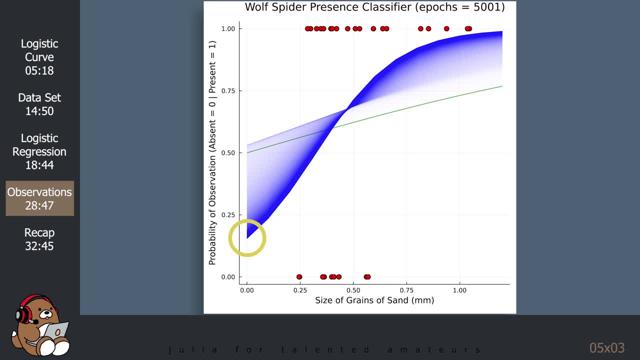 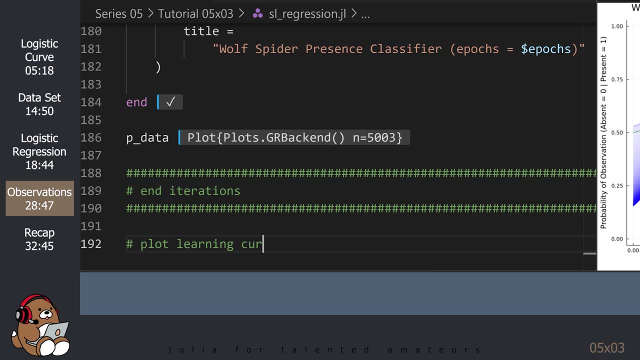 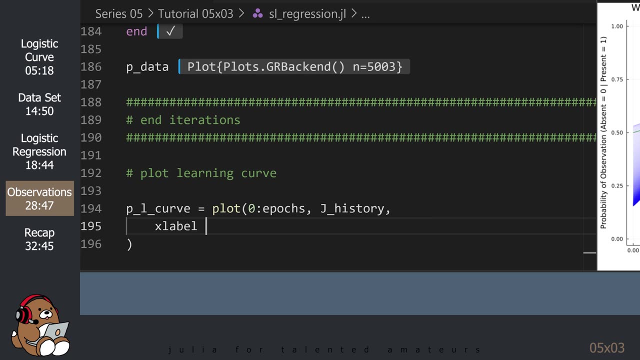 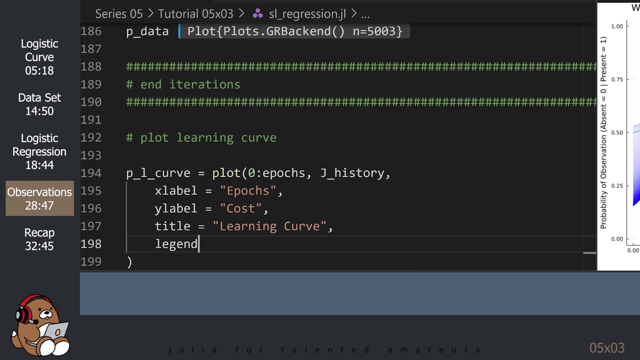 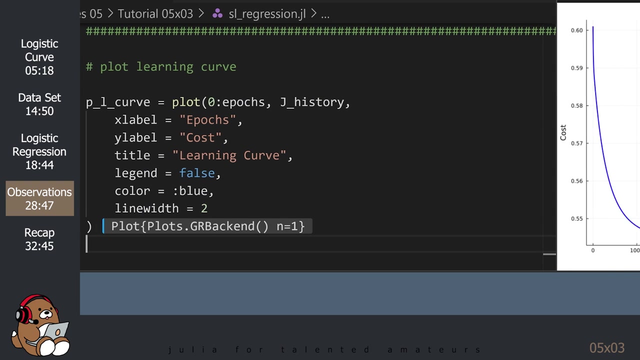 That's because, based on this data, there's always some chance that there may be a wolf spider present, regardless of the grain size. Let's plot a learning curve to see our computer's journey as it went through this process. The values along the y-axis are not important, but the overall shape of the curve is important. 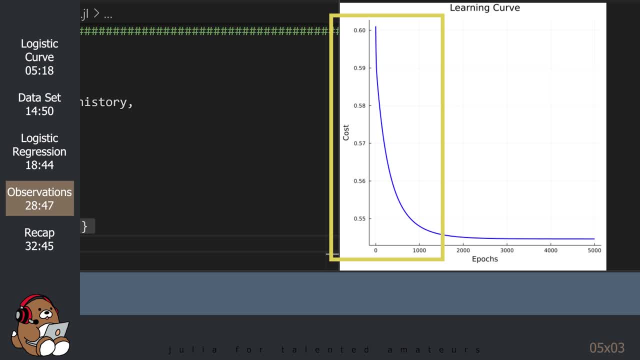 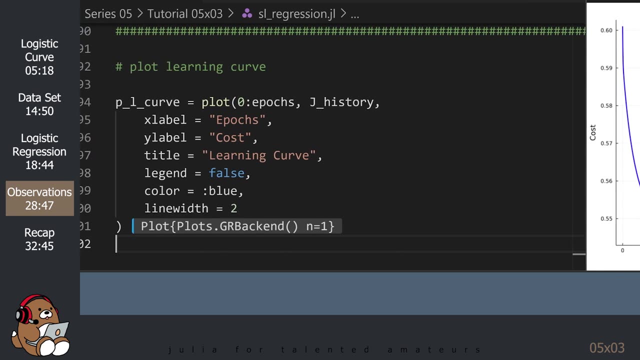 This learning curve shows that our computer was able to make significant improvements to the cost in their early iterations, but the improvements slowed down significantly after 2,000 epochs. This is consistent with what we saw visually. Next let's plot the journey that the parameters went through during this process. 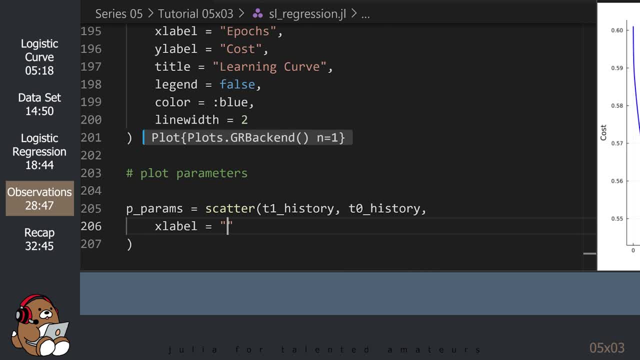 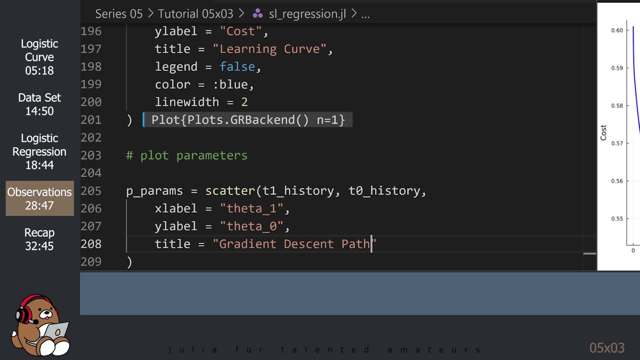 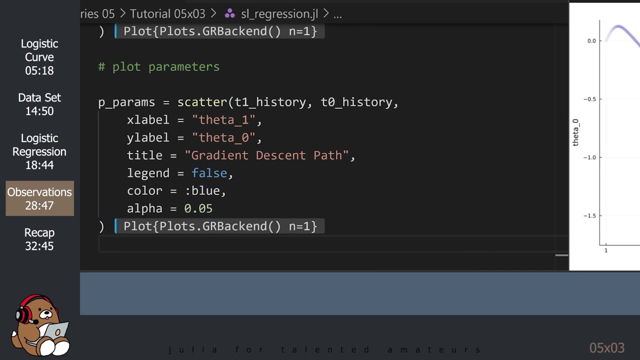 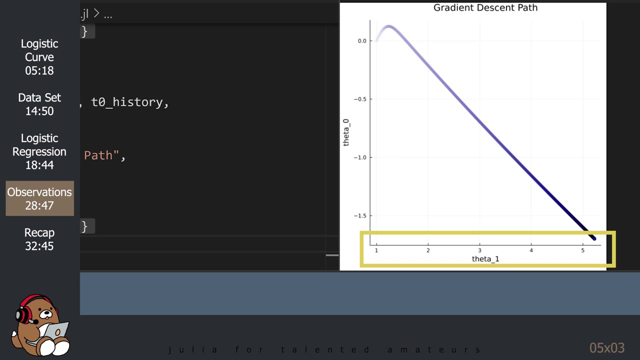 This is a new plot. We did not plot this last week. The data we used to calculate this model was the function that was used to calculate how much of the grain size the tree has across the map. I slowed it down to about 22.7.. As a reminder, theta zero is like the y-intercept and theta one is like the slope. The parameters started their journey in the upper left corner, with theta zero equal to zero and theta one equal to one. This allows me to plot the journey with all the parameters together. 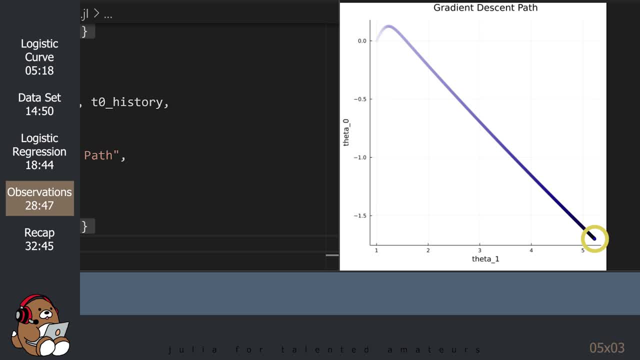 Again, I'm tenant away from the first one. I can't see the pattern of the graph, but it's all the same. Their journey ended in the lower right corner, Just like we saw. visually. this plot shows that the Y-intercept increased initially. 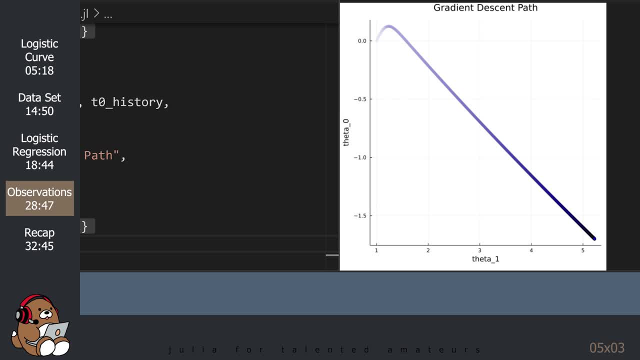 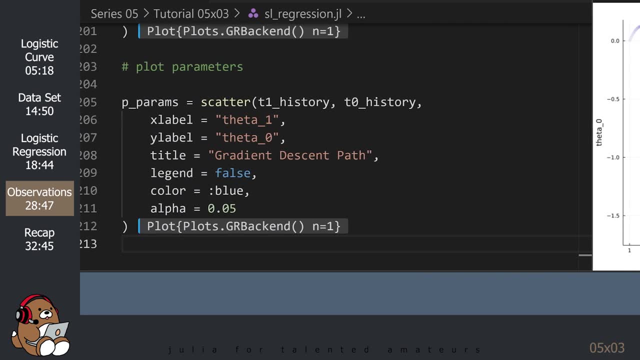 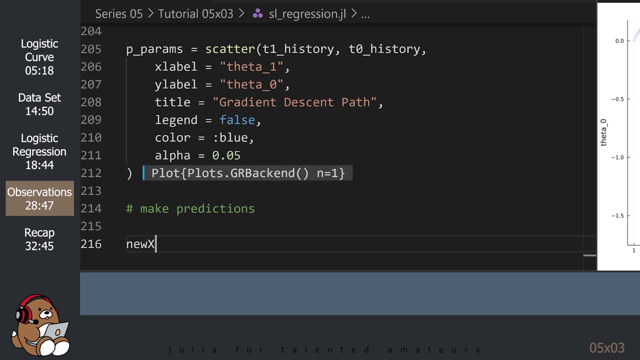 but eventually began to move down. On the other hand, the slope continued to increase with each iteration. Now that we have a working model, let's use it to make some predictions Based on grain sizes of 0.25 mm, 0.5 mm, 0.75 mm and 1 mm. what is the probability of a 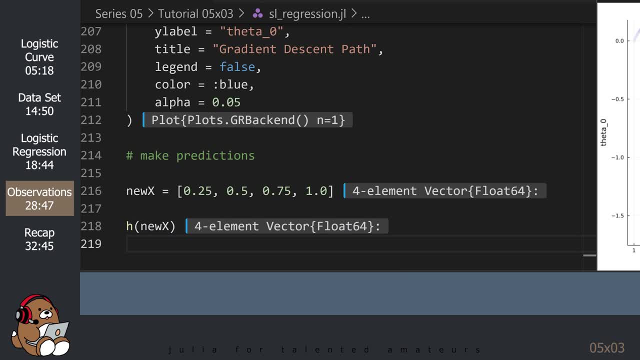 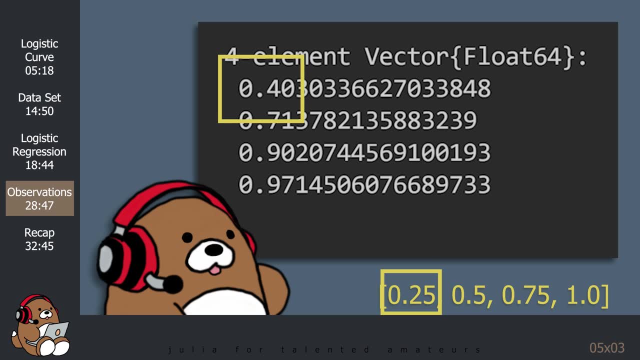 wolf spider being present. The output is in the REPL, So, based on this machine learning generated model, the probability of a wolf spider being present when the grain size is 0.25 mm is 0.25 mm. At the other extreme, when the grain size is 1 mm, the probability of a wolf spider 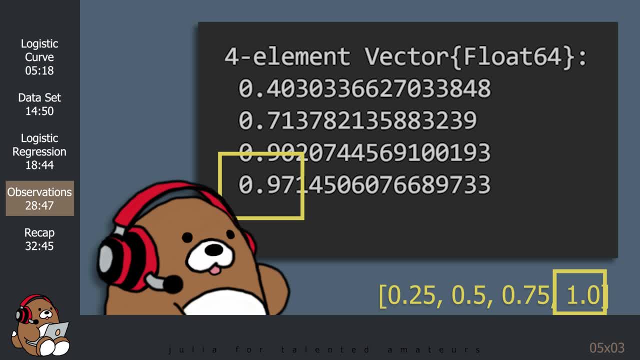 being present is around 97%. It's useful to see the actual probabilities, but since this is a classification problem, you may want to set up some rules to define the decision boundary for the classes. For example, you may want to say that if the probability 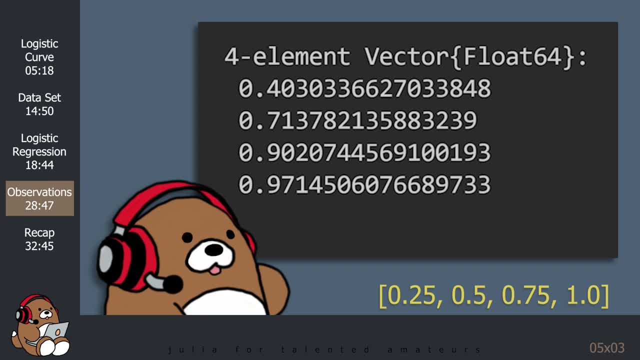 is greater than or equal to 50%, then the result is a positive class. Otherwise the result is a negative class. So in our example, the class is negative when the grain size is 0.25 mm and the class is positive for the larger sizes. Pretty cool, right. 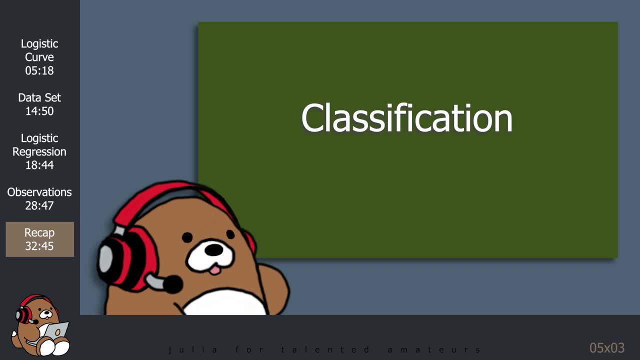 Today we continue to explore supervised learning by getting an introduction to the other major subfield of supervised learning called Classification. Specifically, we learned about the Logistic Regression algorithm. Now that we know the basics of Linear Regression and Logistic Regression, what are some of the key takeaways? 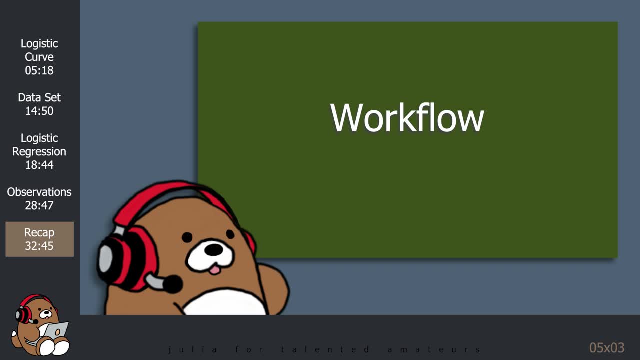 Well, the machine learning workflow for solving both Linear Regression problems and Logistic Regression problems is the same. The only things we needed to change were the Hypothesis Function and the Cost Function In terms of outputs. with Linear Regression, you're trying to create a model that predicts a continuous output.